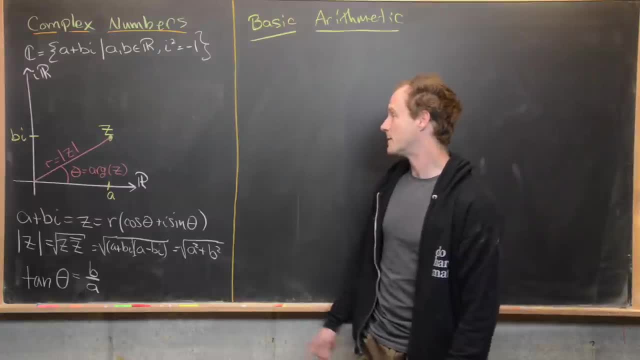 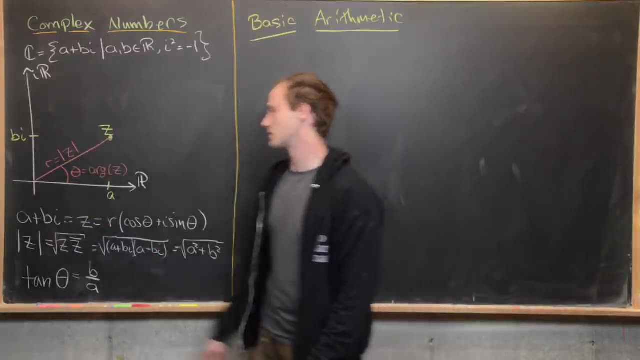 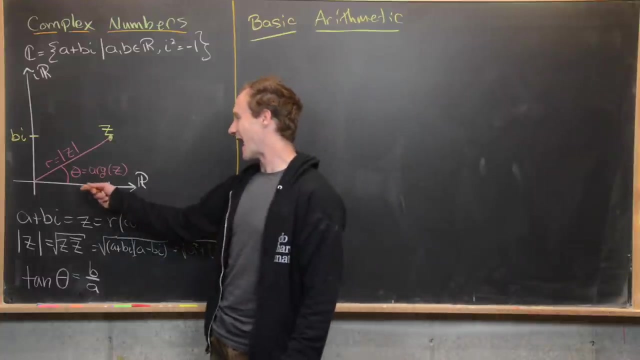 cosine theta plus i sine theta. And here r is called the modulus of the complex number. In other words, that's the distance of this complex number from the origin, And theta is called the argument of this complex number. So that's the angle that is made. 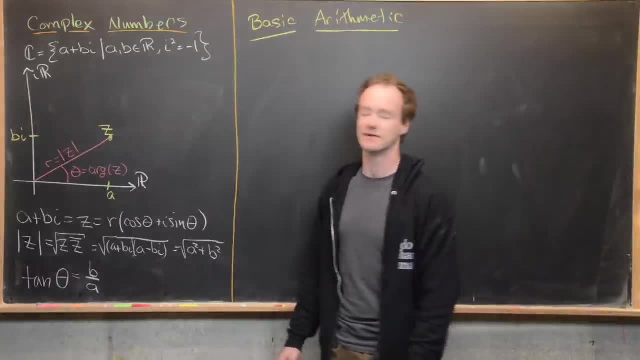 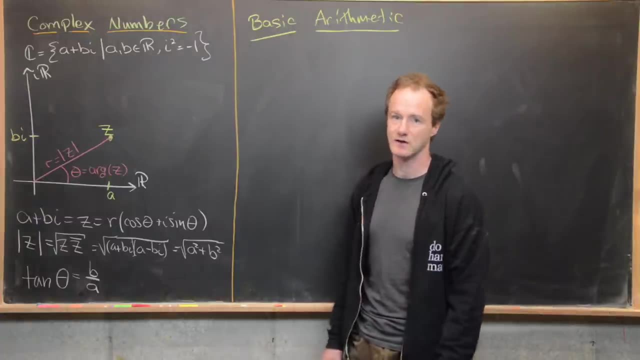 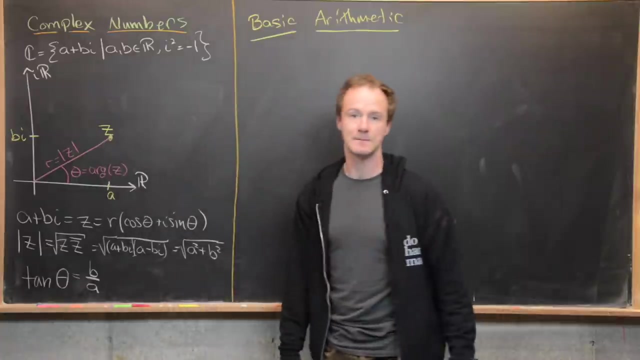 by the ray defined by this complex number and the positive real axis, And we've got some connection between this argument and this modulus. and then the rectangular parts of the complex number as well, And those go like this: So the modulus of z, that's the same thing as the square root of z, times, something. 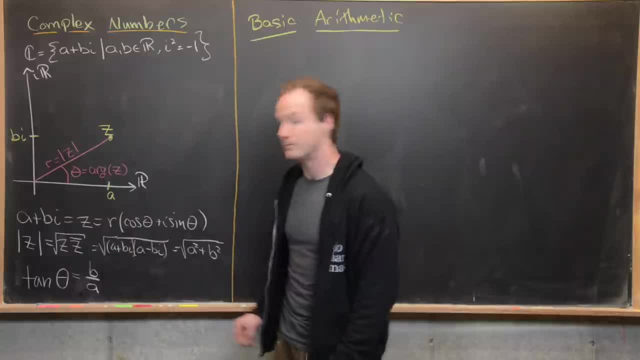 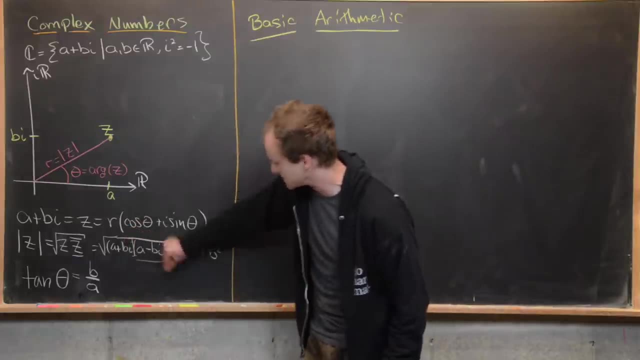 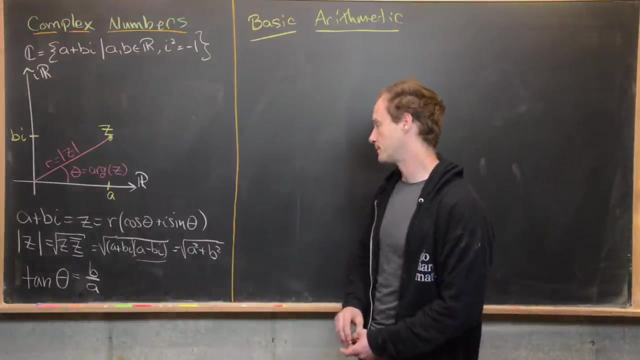 called the conjugate Of z, which I'm going to go ahead and build this into the definition. So the conjugate of z, which I've underlined there in purple, is this a minus bi. So it's almost the same complex number, except we have negated the imaginary part. But notice, if you do this, 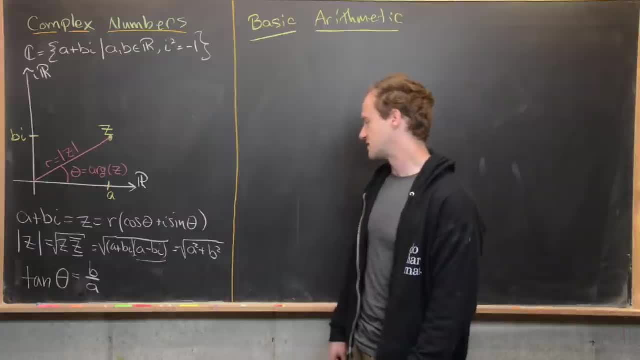 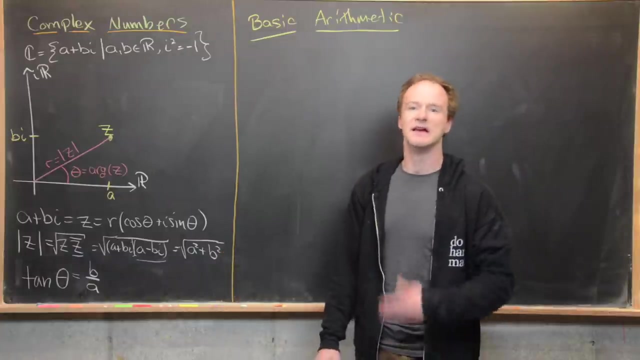 kind of arithmetic application. you'll get this sum of squares, a squared, plus b squared. Notice the cross terms, cancel and then you're left with minus b squared times. i squared, But i squared is minus one. So there we've got this like modulus of the complex number. 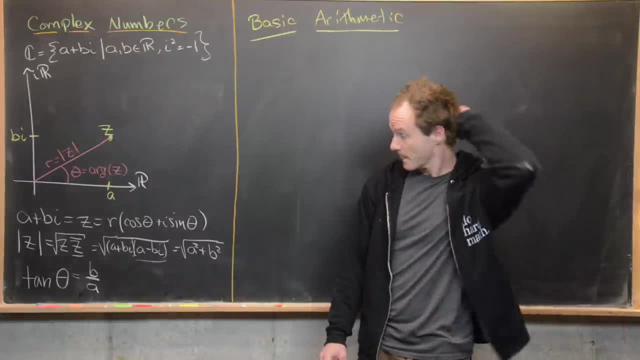 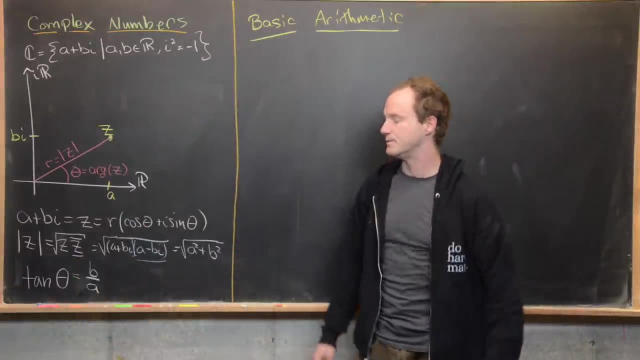 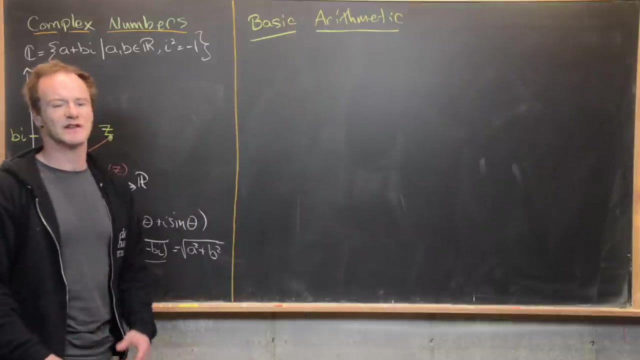 is given by this thing that looks a lot like Pythagorean Theorem. And then next the argument of the complex number. theta has this relationship. that tangent of theta is b over a. Okay, good, So now I want to do some basic arithmetic operations on the complex numbers. 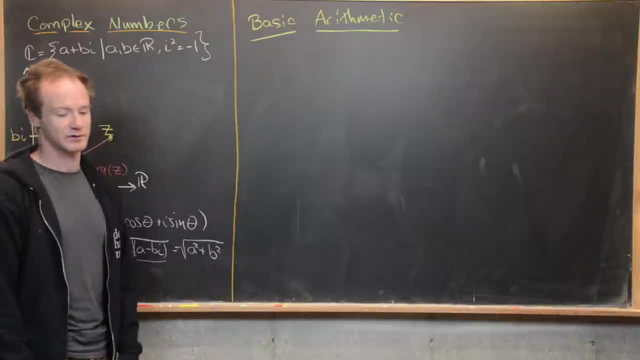 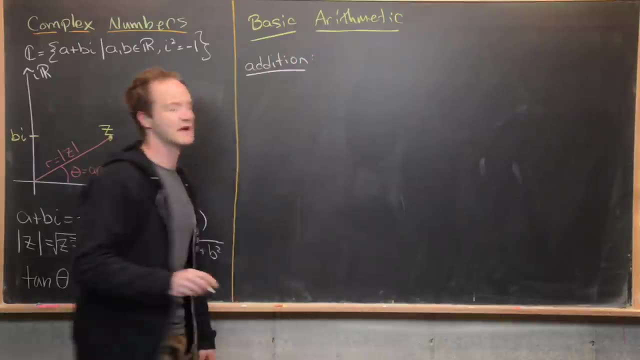 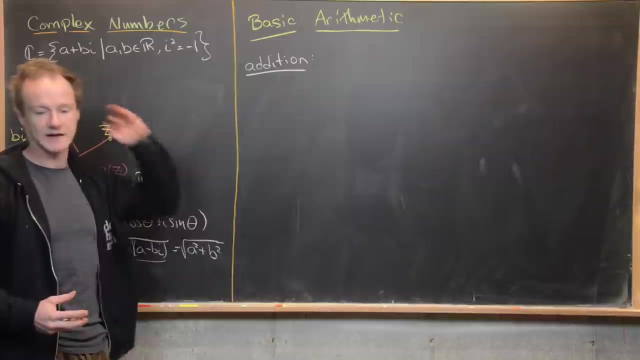 first before we go into looking at contest problem examples. So maybe first we'll look at addition And really we want to think about complex number addition as just really combining things with like terms, But also we can think about it geometrically as a sum. 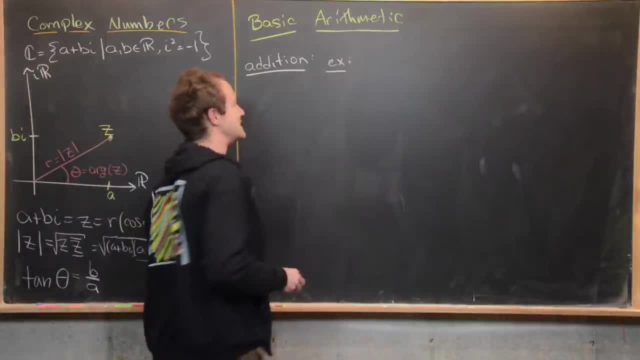 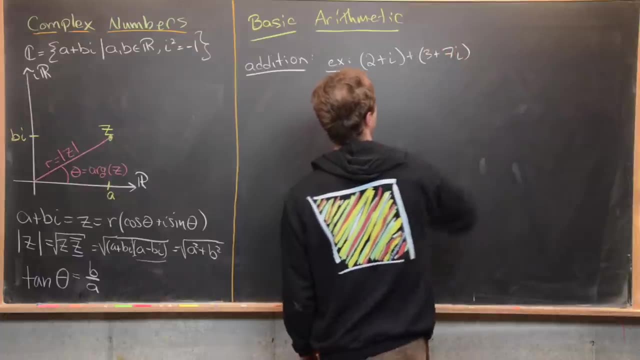 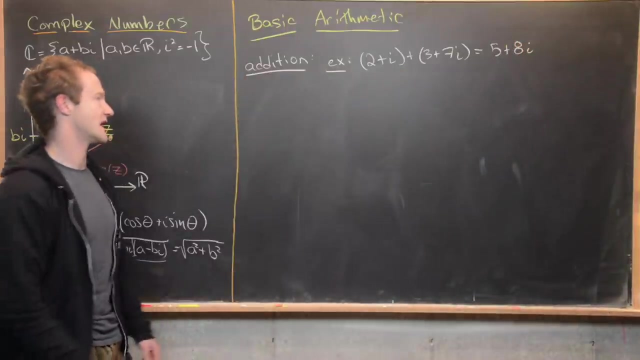 of vectors. So maybe just a very naive example would be something like this: What if we took two plus i and we added three plus seven i? So here we would just combine like terms and get five plus eight i, Something like that. But now if we push this into the complex plane and look at what's, 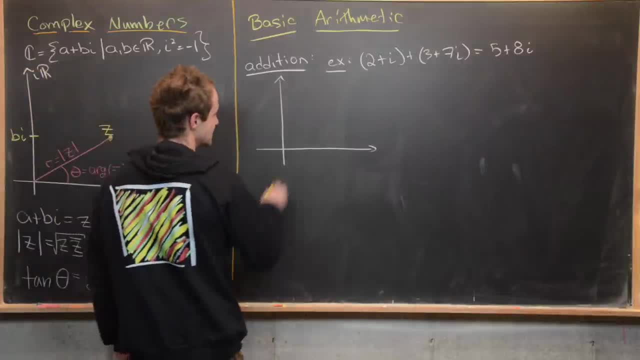 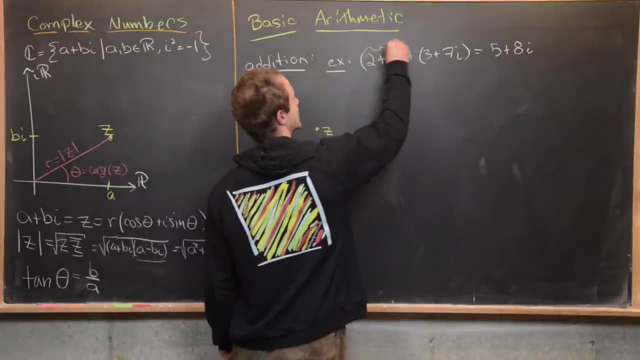 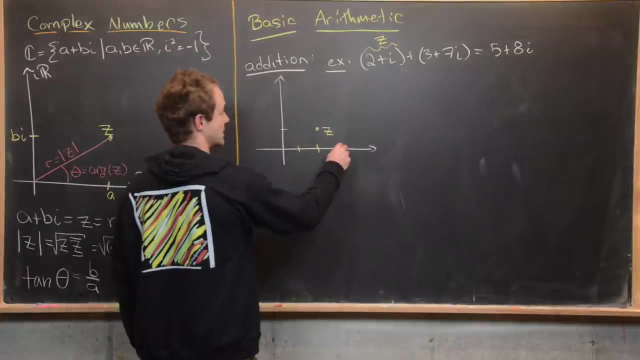 happening. geometrically it's a little bit more interesting. So notice: two plus i is maybe this point right here, which I'll call z, So let's again maybe call this thing up here: z And then three plus seven i. So that's going to be out here. three and then seven. 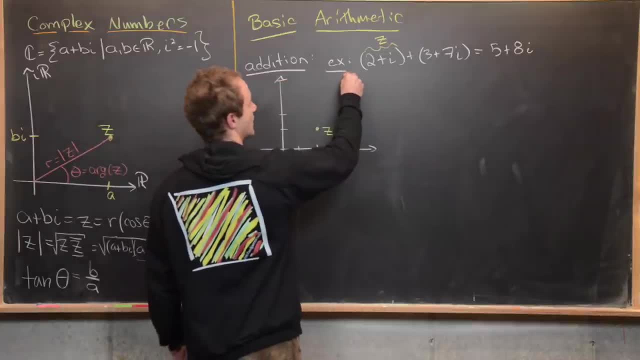 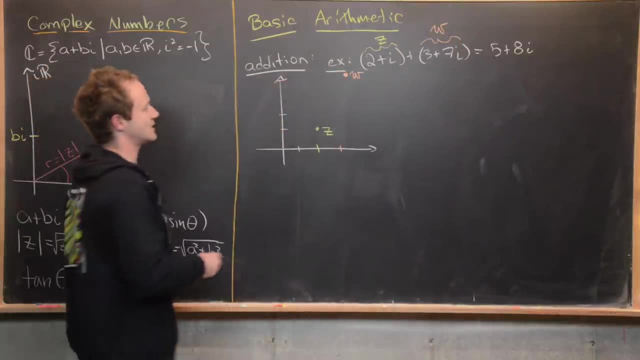 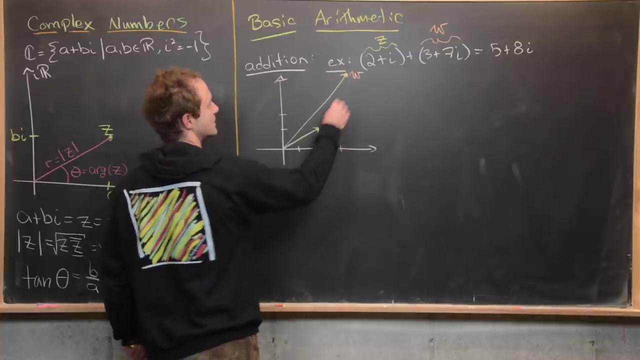 So that's way up here. Maybe we'll call this point here: w. And now what do we get when we add those? Well, it's like completing a parallelogram. So this would be like z, This would be like w. And then, if we complete this parallelogram, 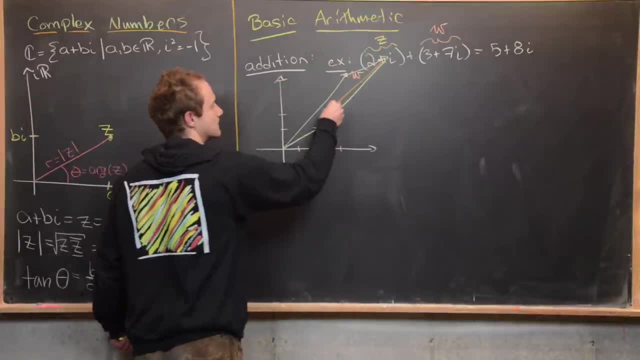 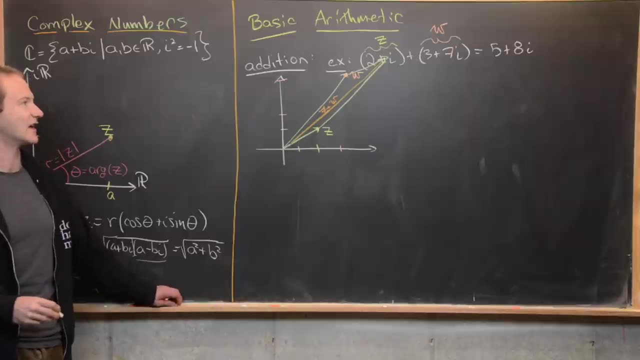 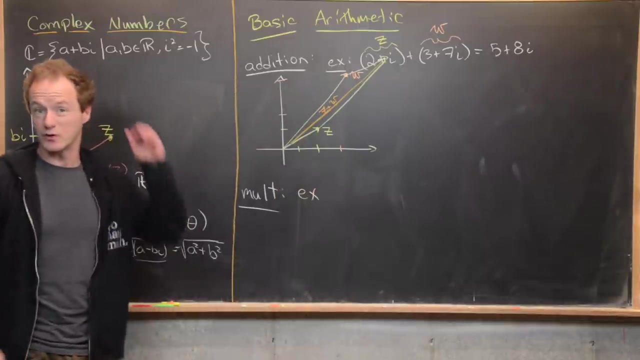 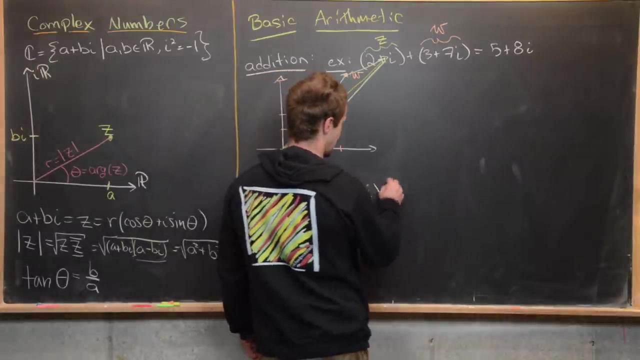 to the end. then the diagonal right, there is z plus w. Okay, good, So just like adding vectors. Now, what about multiplication? Well, again a naive example. you would just like kind of FOIL everything out and then add as necessary, So like if we had three minus, i times four plus, i Say that, So we 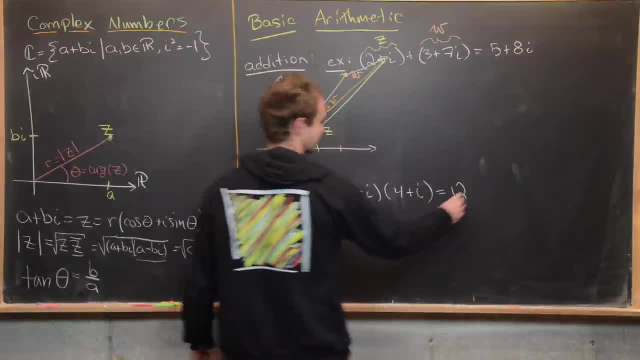 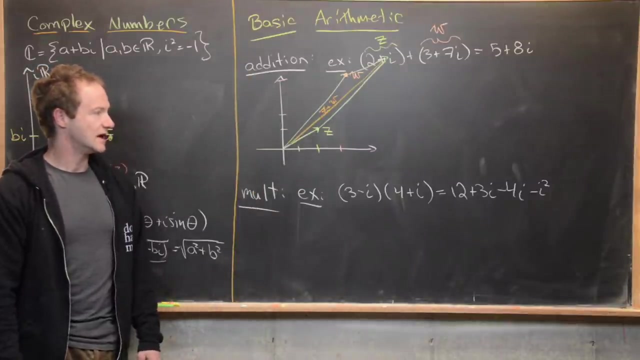 would do three times four. That's going to give us twelve, Three times i. That's going to be plus three i minus four i from the minus i times four. And then we've got minus i times i. So that's going to be minus i squared. But we know minus i squared is going to be positive. 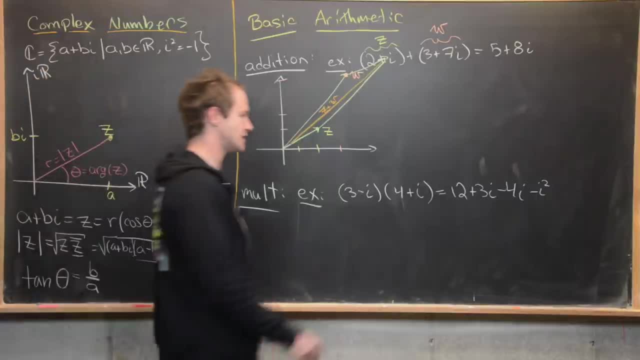 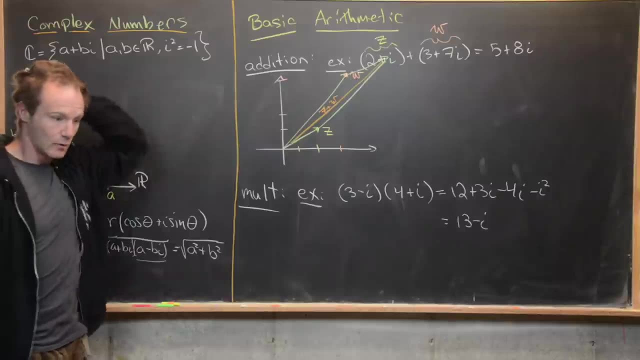 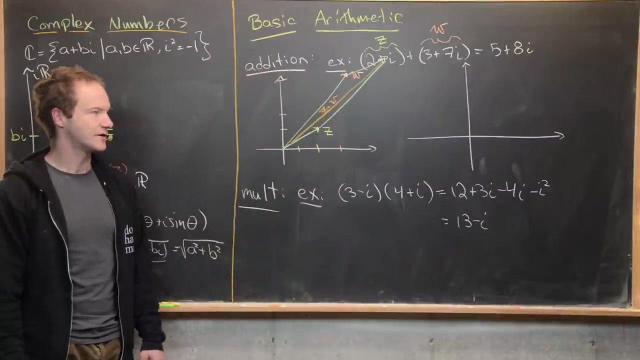 one, because i squared is negative one. So we've got negative, negative one. So that's going to give us thirteen minus i in the end. Okay, great, Now what about a geometric application of multiplication? Well, so if we're multiplying by a real number, let's say a positive, real- 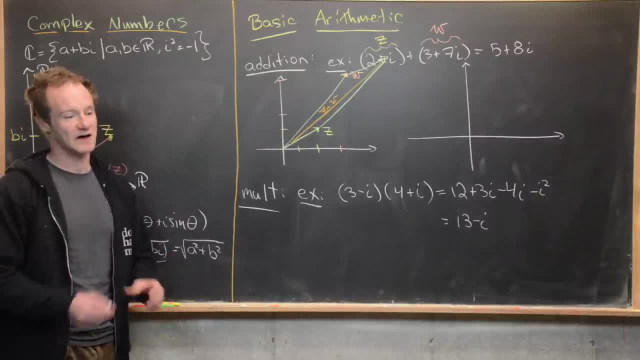 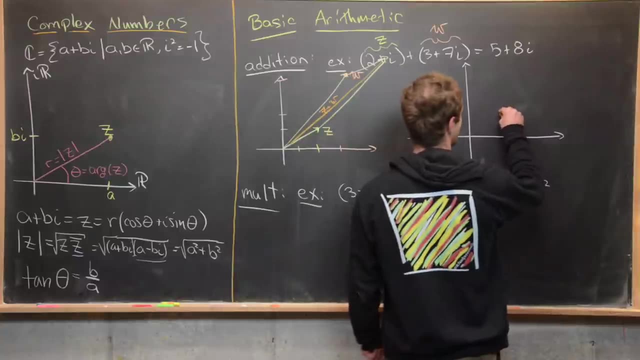 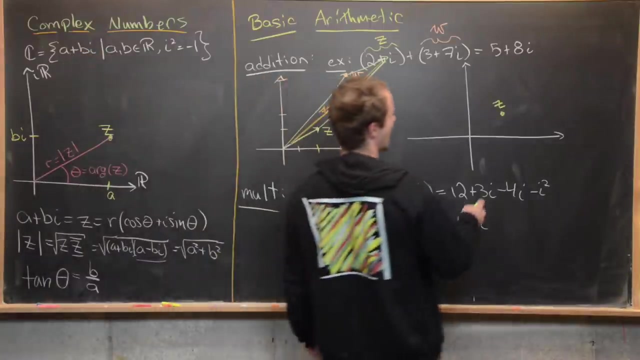 number, then that has the geometric effect Of kind of expanding this plane by a factor of that real number. So let's maybe say that we have z here, like that, And then let's say we multiply by a, And let's say a is like: 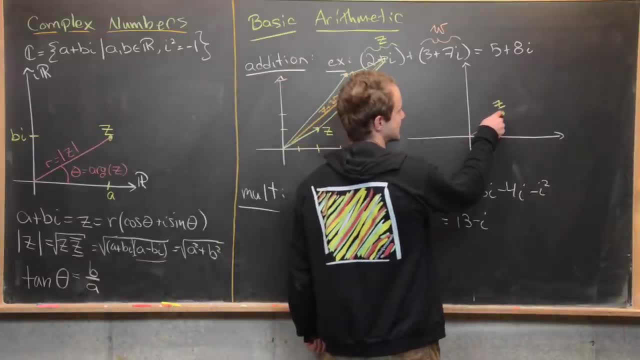 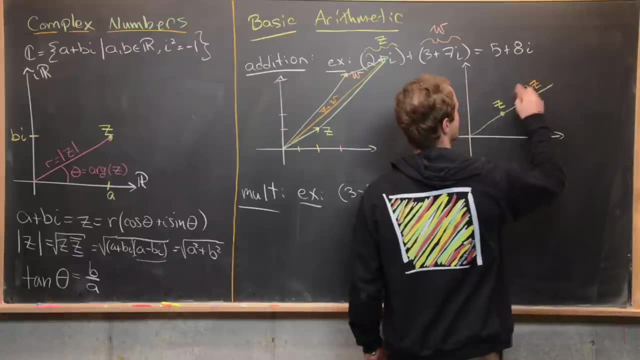 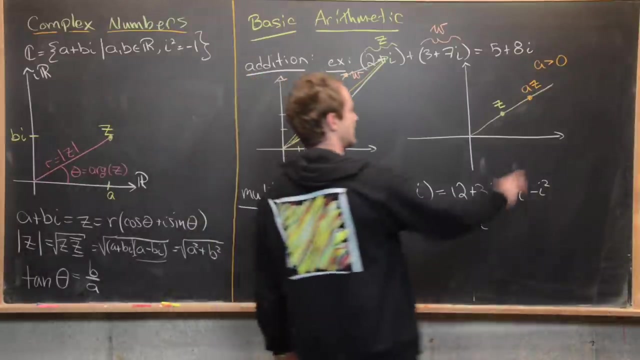 bigger than one. Well, we're going to like complete this ray along z and then we'll get a z out here. And this is here. We're multiplying by a real number which is bigger than zero. So notice, if a is equal to one, we land right back on z If it's bigger than. 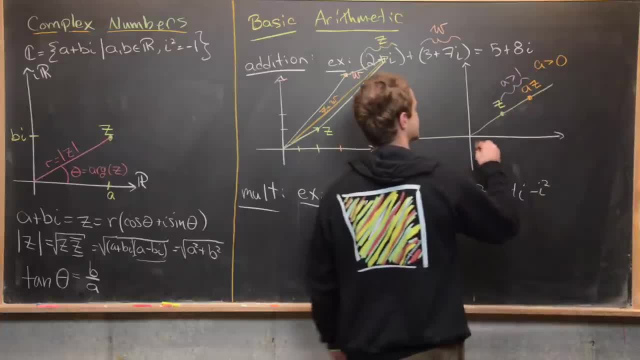 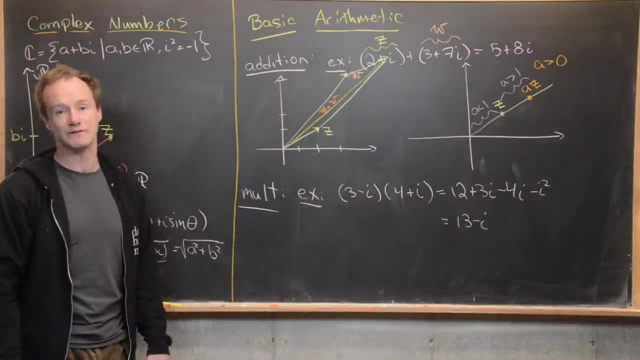 one, well, we're going to land in this direction, And if it's less than one, we're going to land in this direction. So it's an expansion or a contraction of the plane. And then another important case to look at is what if we multiply by something of the form, cosine theta plus? 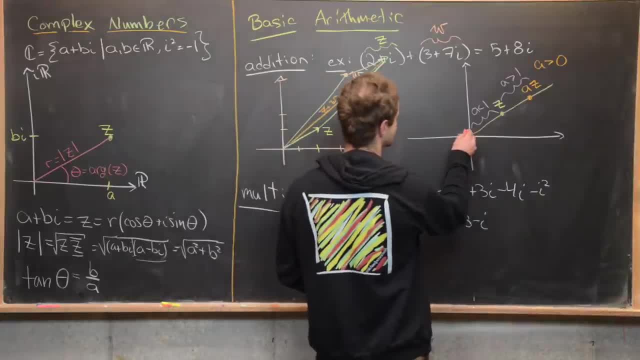 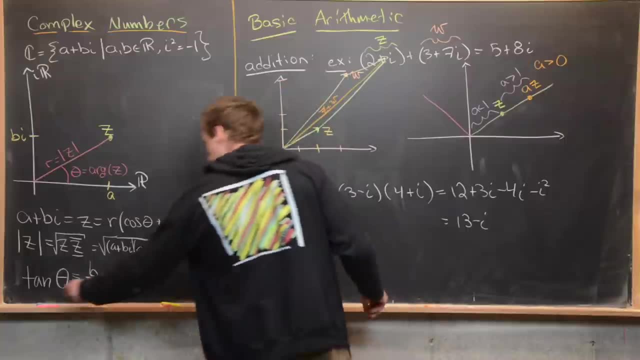 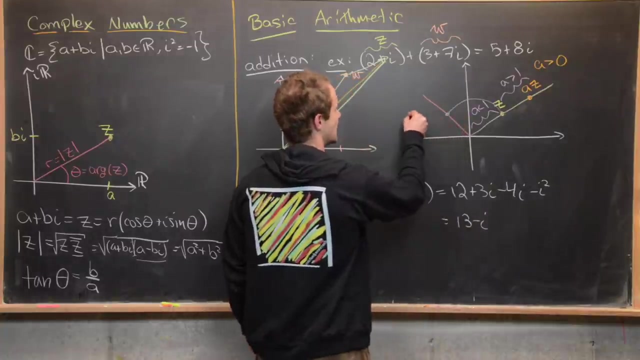 i sine theta, then the modulus stays the same And what we end up doing is just rotating this point. So here we'll make sure we're at the same modulus. And now this point right here is z times cos theta plus i sine theta, And the angle right here is given by theta. 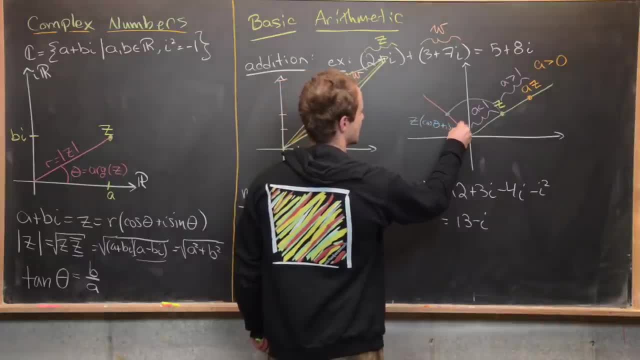 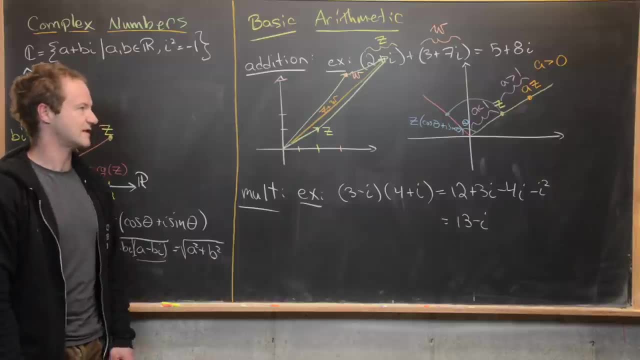 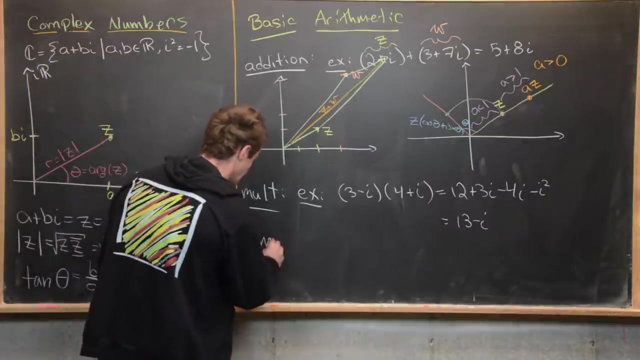 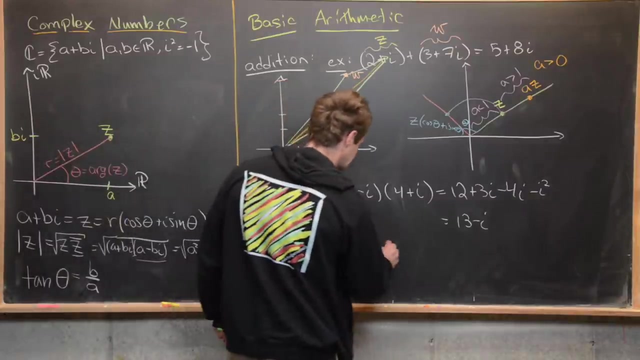 So, in other words, multiplying by a is equal to z times cos theta plus i sine theta, And that's what we end up doing. Multiplying by this cos theta plus i sine theta is the same thing as rotation. Now we can put this all together to say that if we multiply by w, then that expands the plane. 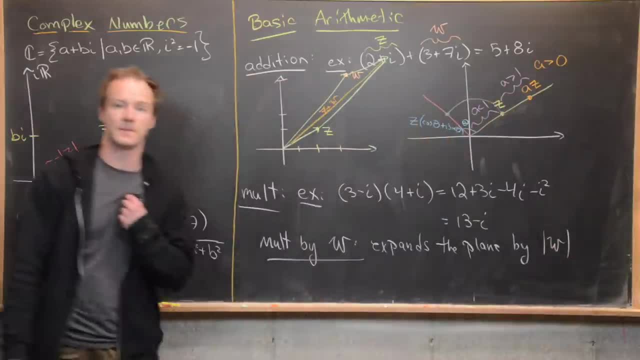 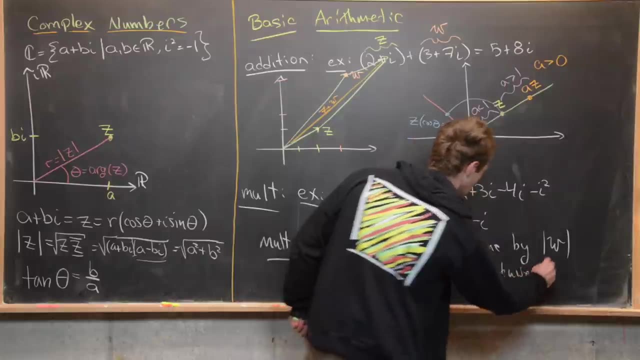 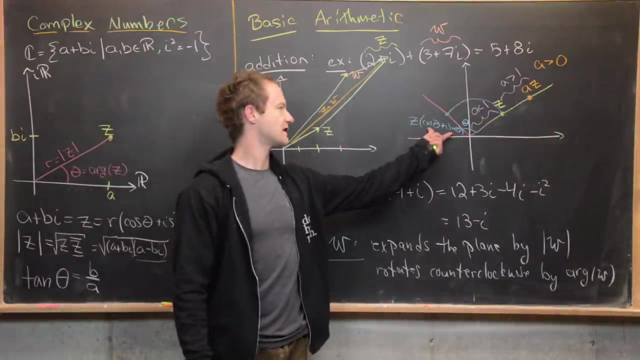 by a factor of the modulus of w, And then it rotates counterclockwise By a factor of the argument of w, Because, notice, all that's really left here is the argument. the modulus of this cosine, theta plus i sine theta, is one, But then all that's. 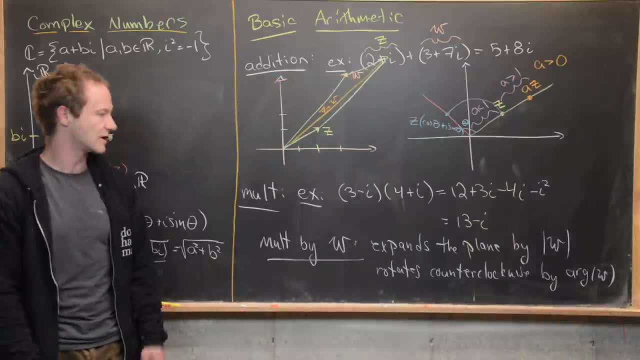 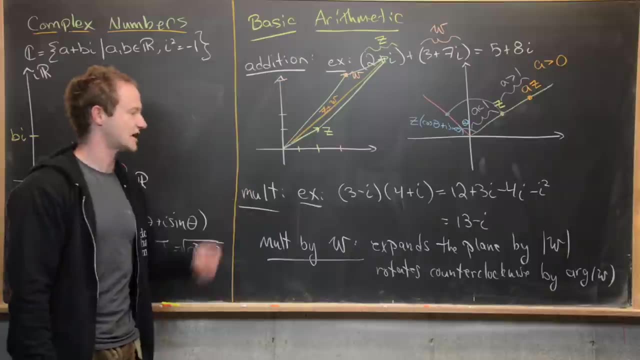 left, in this case, where we have just a, a positive real number, is the modulus of the number. Okay, so that's a nice geometric interpretation of addition and multiplication. I'm going to go ahead and clean this up And we're going to look at how to divide. 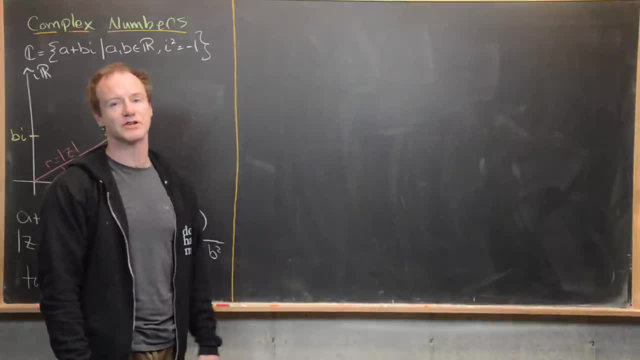 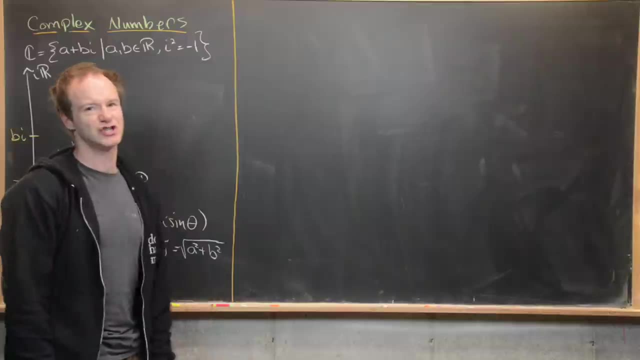 Complex numbers. So now that we've looked at some basic operations on complex numbers, let's talk about division of complex numbers, And I'm going to do this just by a quick example, And then you can generalize this kind of on your own pretty easily. So let's say, we want to take the complex 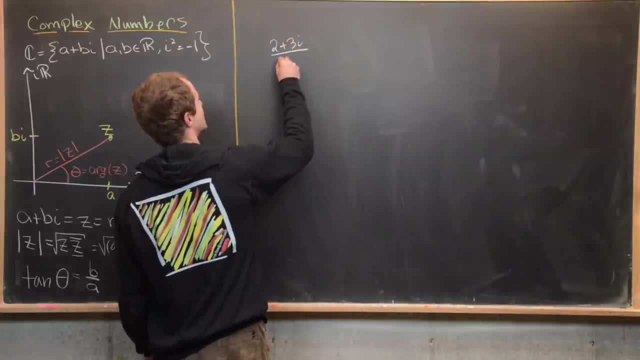 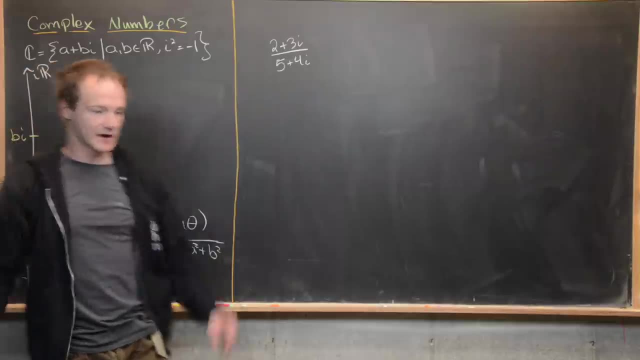 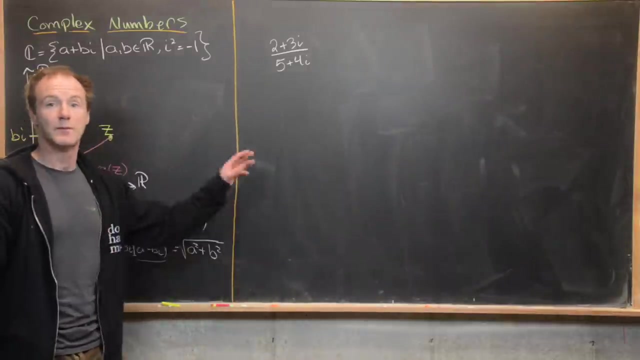 number 2 plus 3i and divide it by the complex number 5 plus 4i. So the problem here is: we know that complex numbers are supposed to be of the form a plus 4i, where a and b are real numbers. But that's not what we have here. But now, using this, 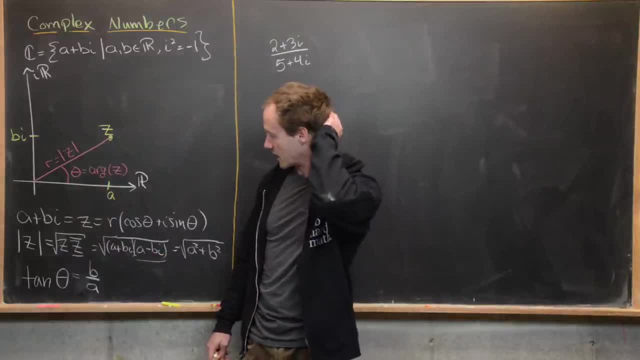 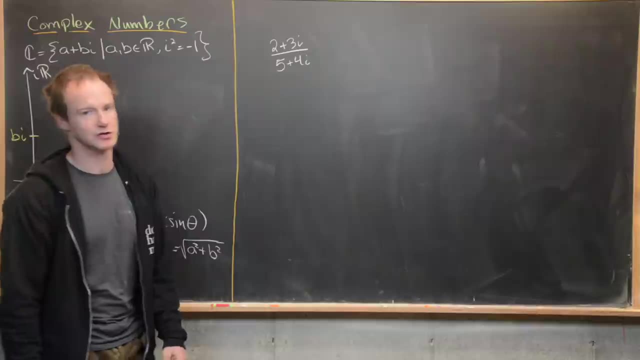 idea of the conjugate which I have under over here, underlined in purple. we can multiply the numerator and the denominator of this fraction by something that turns the denominator into a real number, which is exactly what we want to do. So let's group these Multiply. 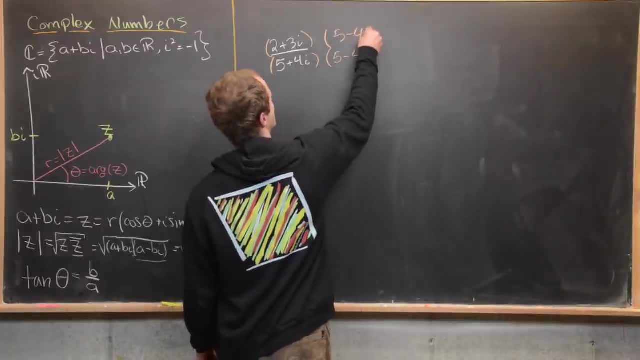 the numerator and the denominator by 5 minus 4i, And I want to point out that 5 plus 4i and 5 minus 4i are real numbers And that's exactly what we want to do. So let's group. 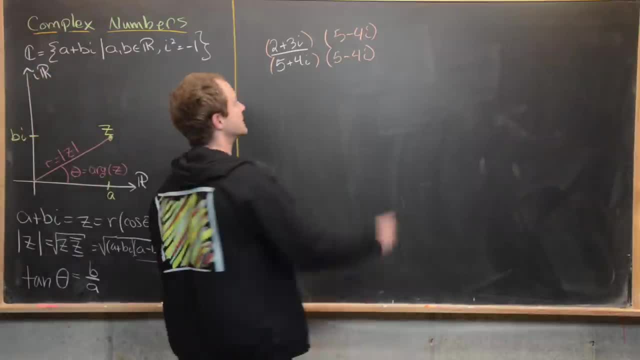 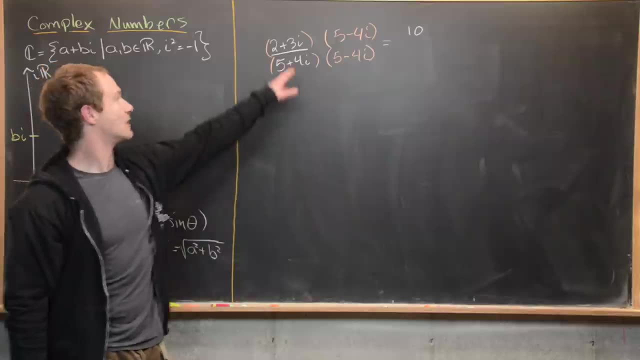 these complex conjugates of you that each other. so let's see what we get here. so this numerator, so that's gonna give us 10 from the 2 times 5, and then we're gonna have plus 12. so that's our real part. notice: we have minus 12, I squared. 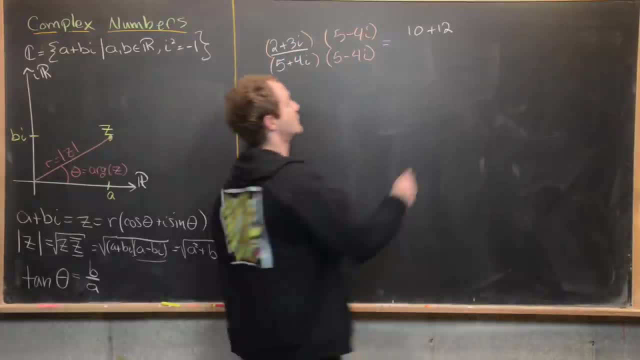 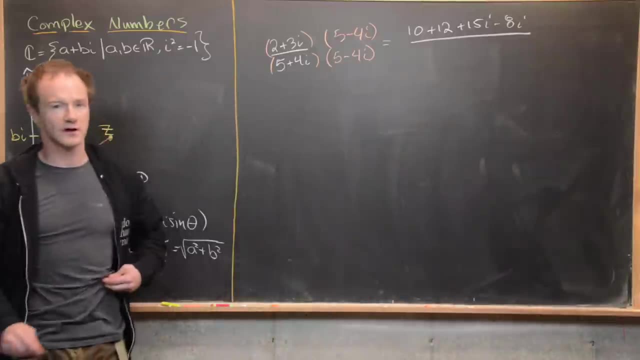 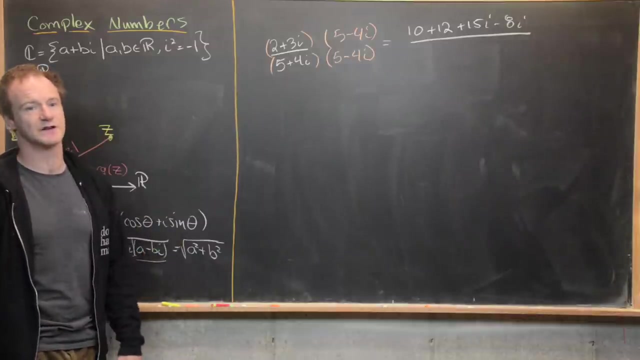 but that's gonna be plus 12, and then next we have plus 15 I and then minus 8 I. so that's what we have in the numerator. then the denominator is even easier because we've got this like difference of squares thing happening, but one of our squares involved involves I, so that really turns into a sum of. 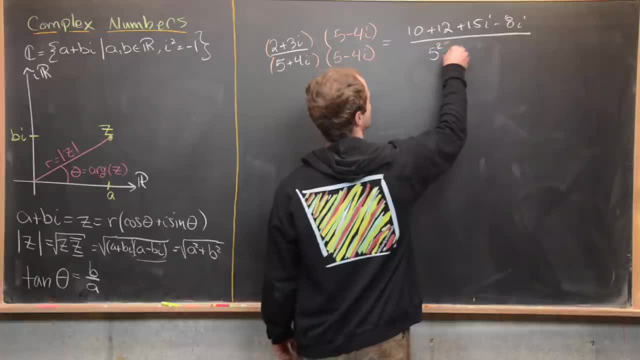 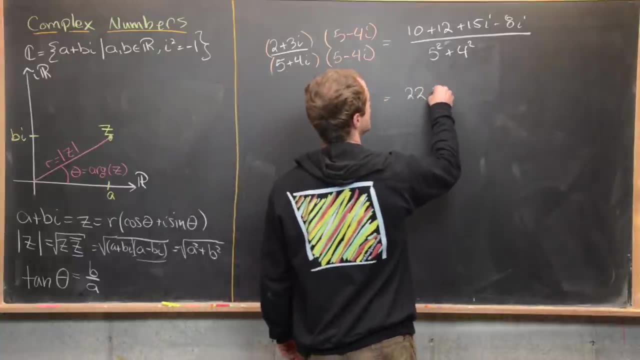 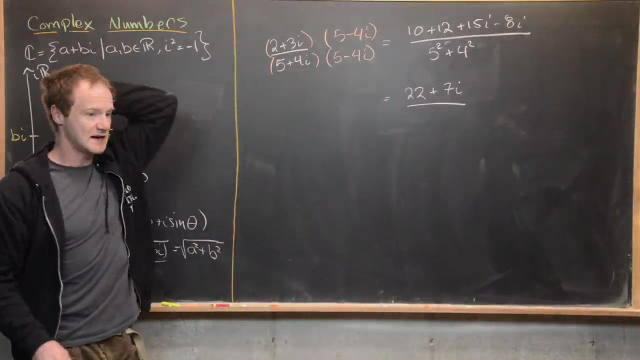 squares, so this is going to turn into 5 squared plus 4 squared after multiplying everything out. okay, so let's see, in the end we're gonna have 22 plus so 7 I all over, so that's 25 plus 16. so let's see, 25 plus 16 is 41, like that. 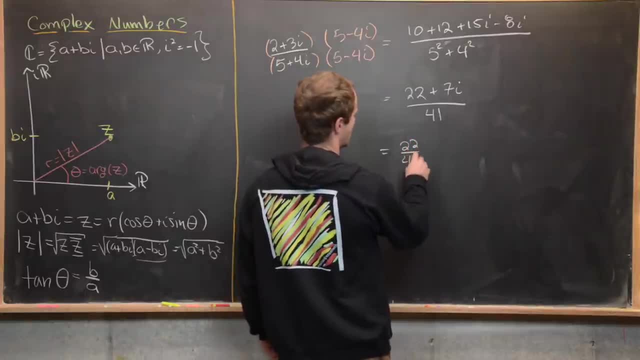 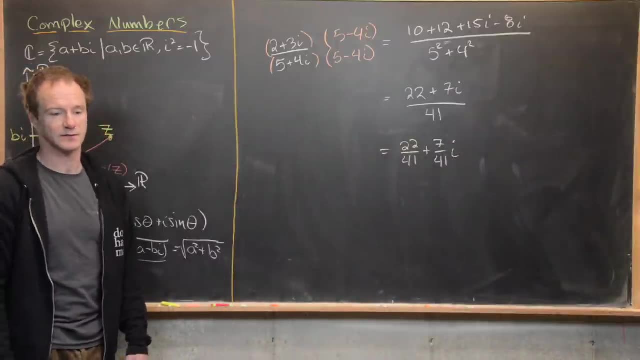 and then we're gonna have 12 squared plus 4 squared, so that's 25 plus 16. so that's, but now maybe we want to write this as 22 over 41 plus 7 over 41 I, so that would be like the quotient of those two complex numbers. okay, so let's maybe clean. 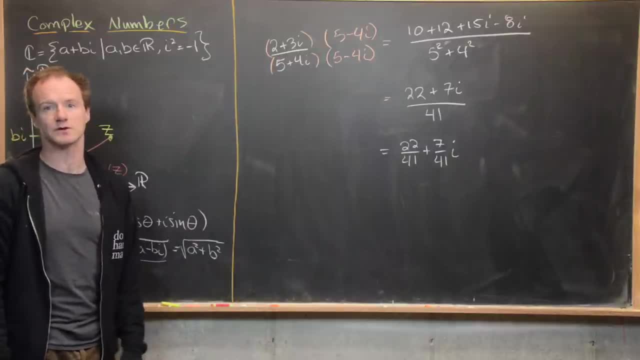 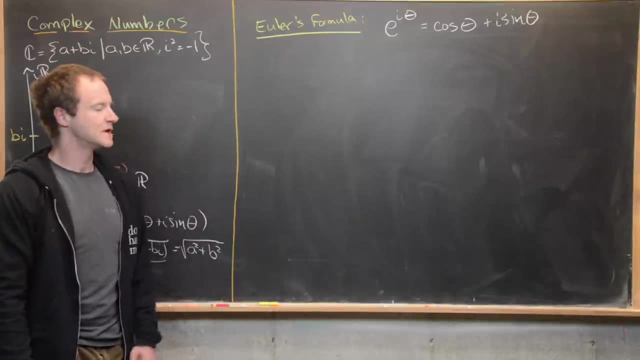 up the board and then we're gonna look at some really important formula known as Euler's formula. okay, so the last basic thing that we need to look at before we go into some examples is something called Euler's formula. you can derive Euler's formula number different ways. 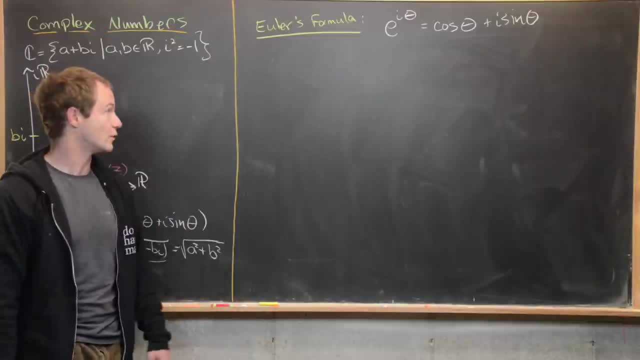 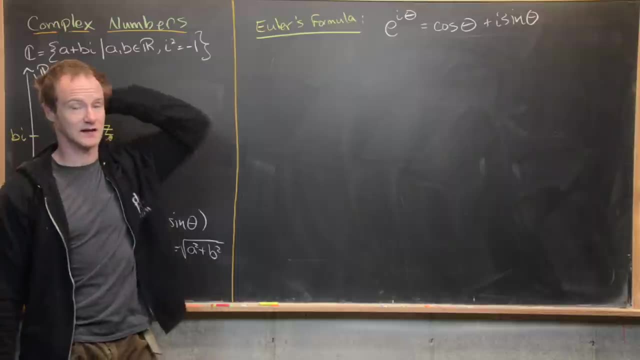 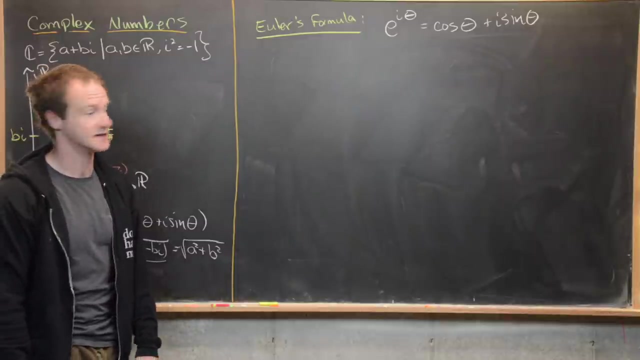 I'll let you guys maybe check the details on this however you want to, but what you end up with is e to the i theta is equal to cosine theta plus i sine theta. so if you've got a complex exponential like this, it can be broken down into cosines and sines. so let's maybe like look at a quick example. 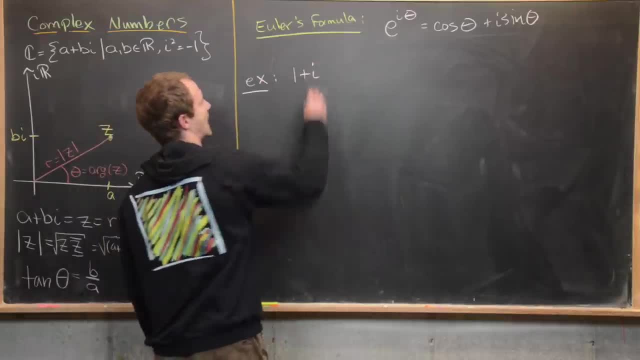 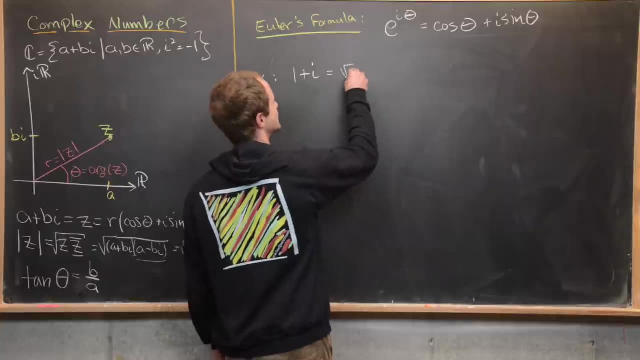 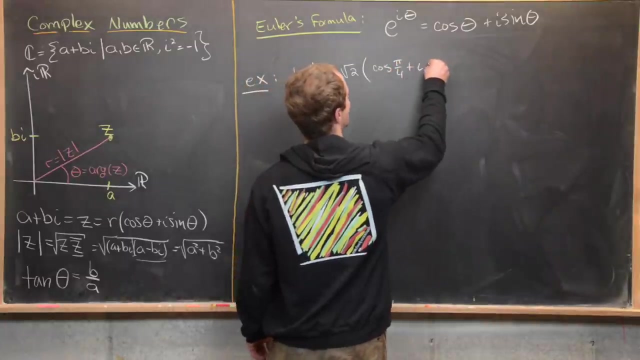 of this. notice, if we have 1 plus i, then that's going to be equal to. well, notice the modulus of this: is the square root of 2, so we have the square root of 2 and then we have cosine of pi over 4 plus i, sine pi over 4. now notice the cosine of. 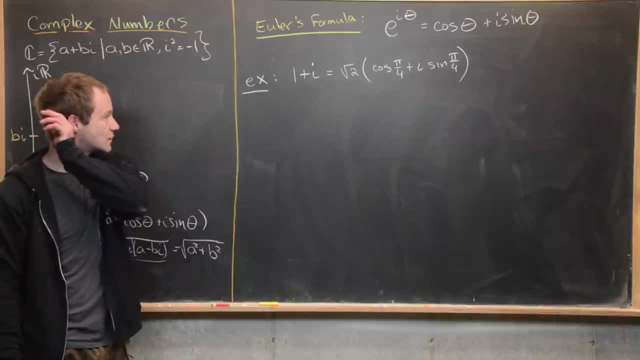 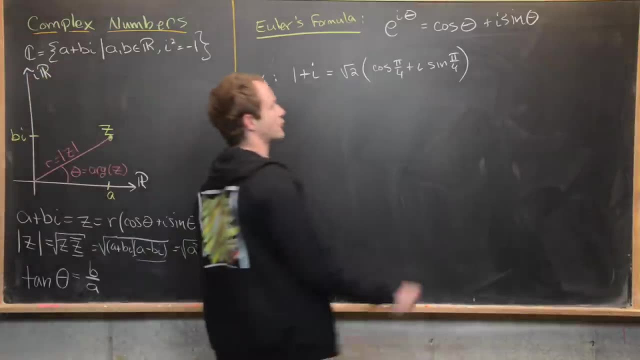 pi over 4 is 1 over root 2 and sine pi over 4 is also 1 over root 2. so if you multiply the root 2 through, that cancels. but this is our bridge to write this in polar form. so now we can write this as square root of 2 times e to the i pi. 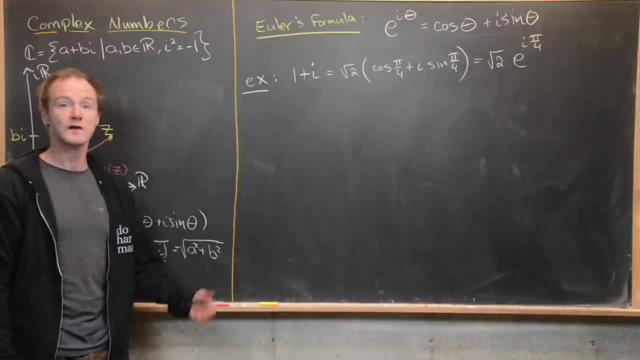 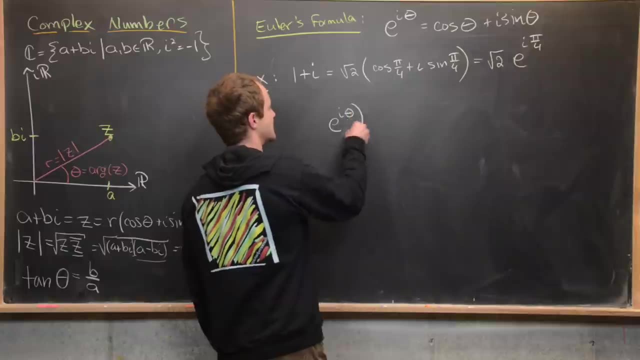 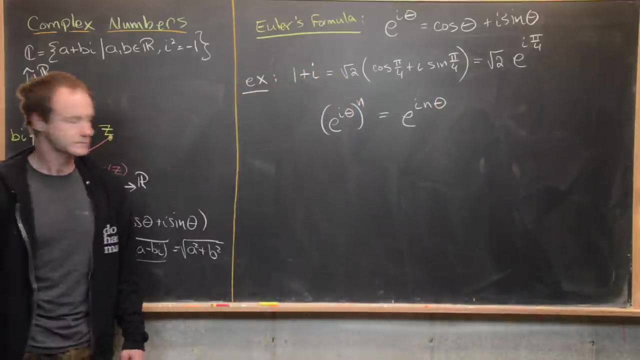 over 4 using Euler's formula. Euler's formula is also a quick bridge to find some trig identities, like, for instance, if we take e to the i theta and we raise that to the nth power by exponent rules, we know that that's e to the i in theta, but then applying Euler's 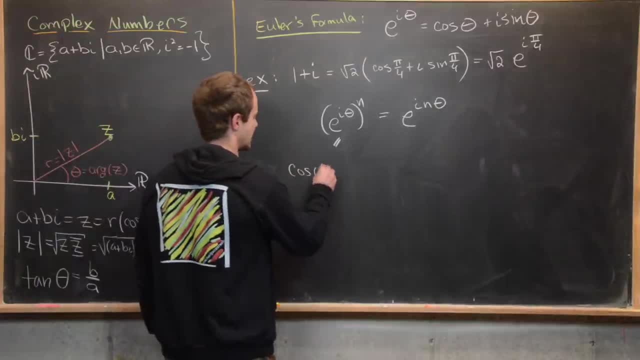 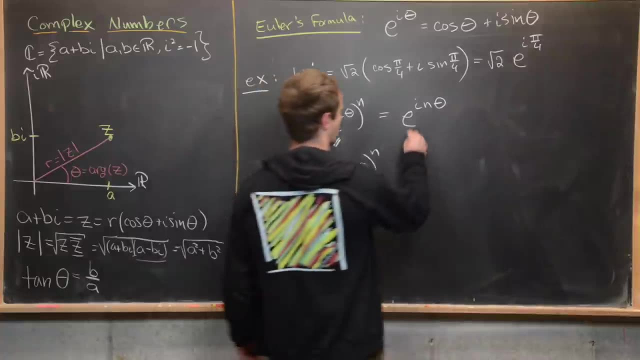 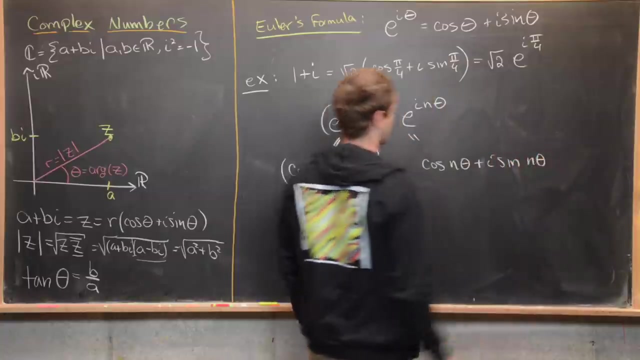 formula to both sides of this. we end up with cosine theta plus i sine theta. all to the nth power on the left hand side, and then on the right hand side we end up with cosine of n theta plus i sine of n theta. then we can expand this for whichever n that we're. 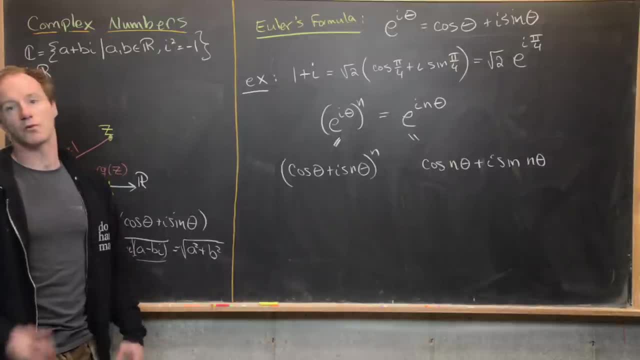 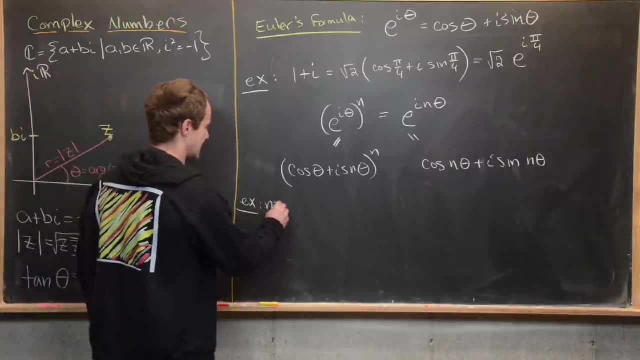 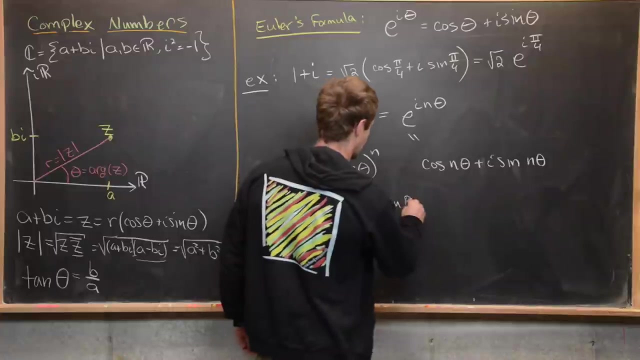 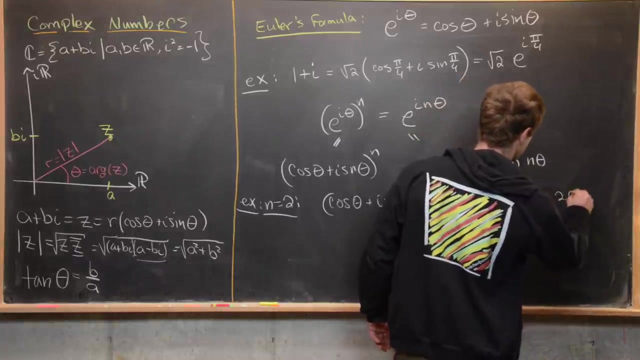 interested in and then extract real or imaginary parts as necessary to come up with some nice trig identities like, let's say, for example, we set n equal to 2, so that's going to give us cosine theta plus i sine theta squared equals cos 2, theta plus i sine 2 times theta. like that: 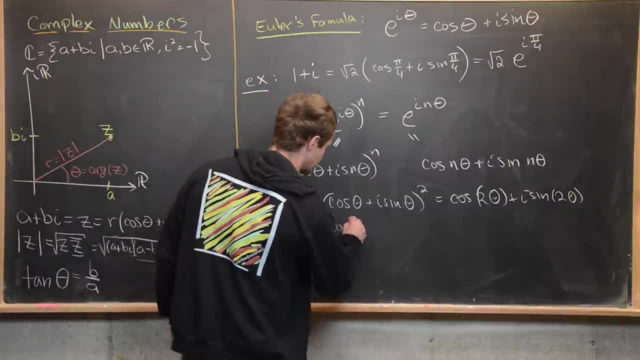 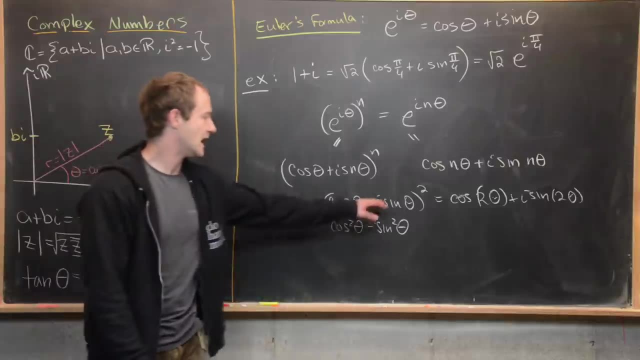 but now we can FOIL out the left hand side. notice: we're going to get cosine squared theta minus sine squared theta. so that's going to be the real part from cosine times cosine, and then i sine, times i sine, and then we've got the cross terms, which are going to be equal to 2. 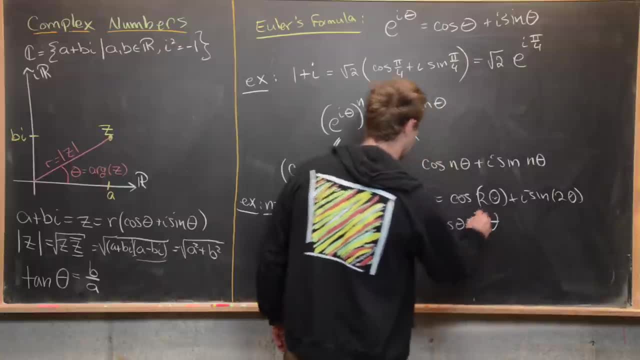 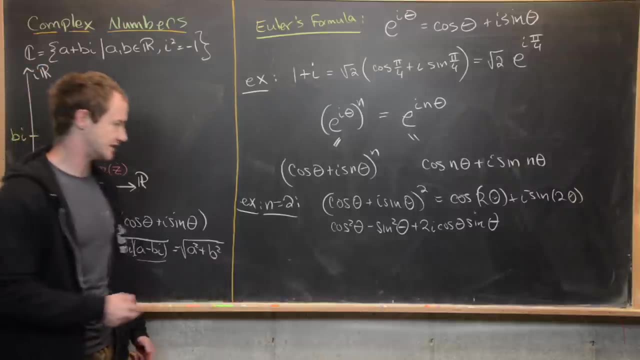 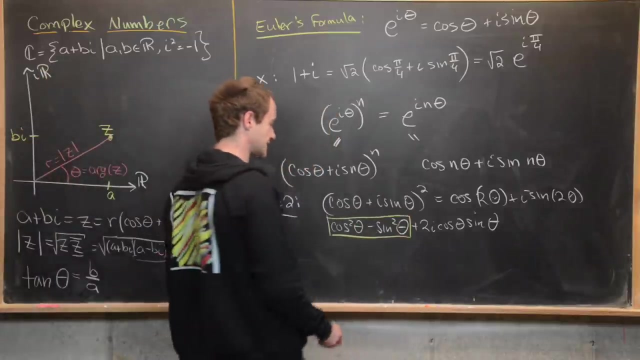 2i: cos theta, times sine theta. But now we can equate the real part on each side of the equation and the imaginary part on each side of the equation, to come up with the well-known trig, double angle identities. So here we've got cosine squared minus sine squared. So that's going to be. 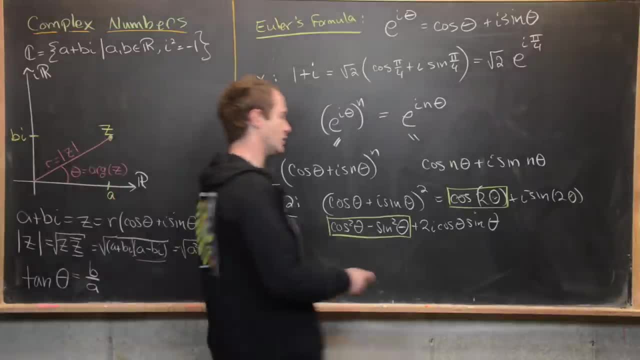 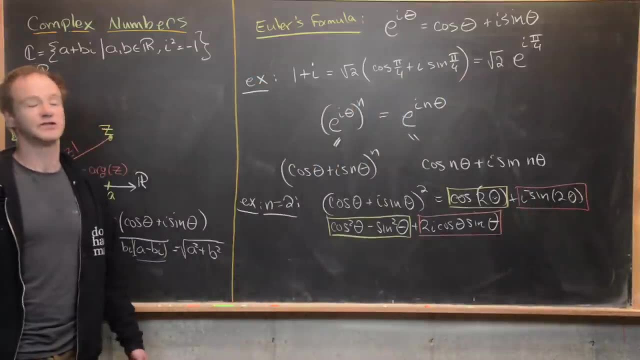 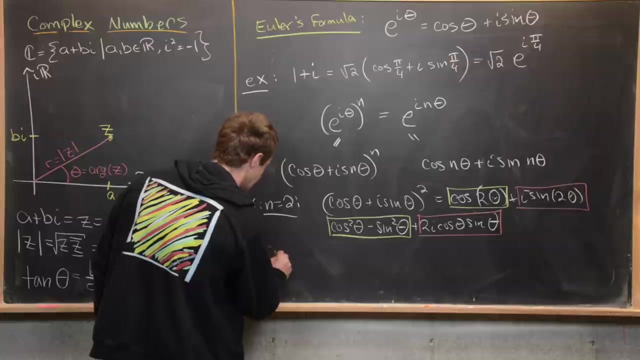 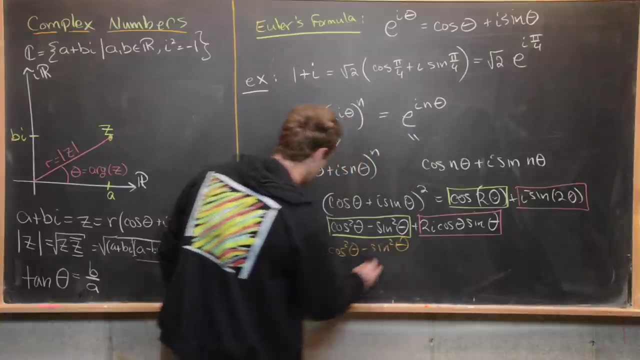 cosine 2 theta, So those two are equal. And then we know that 2i cosine theta sine theta is going to be the same thing as i sine 2 theta, just by extracting real and imaginary parts. So now we can write down that this implies that cos 2 theta equals cos squared theta minus sine squared theta. 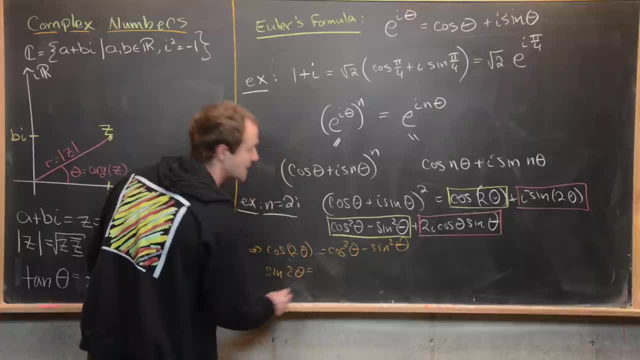 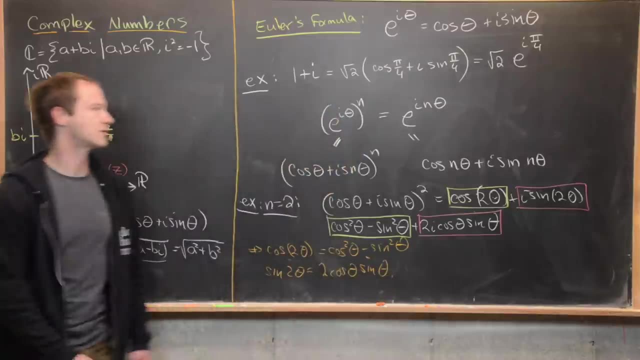 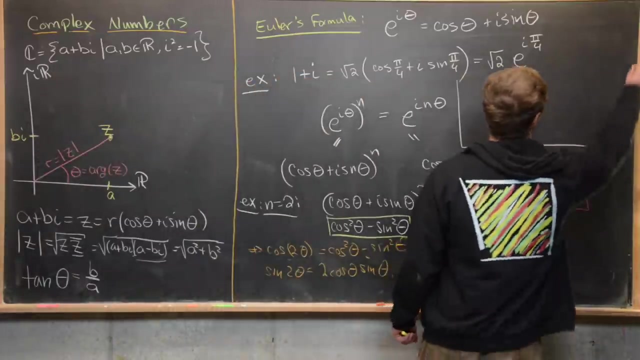 And also that sine 2 theta equals 2 times cos theta times sine theta Great. Now you can even do this by multiplying the real and imaginary parts of the equation. So that's going to be this for different angles. So let's maybe fit that in up here. We can just expand that two. 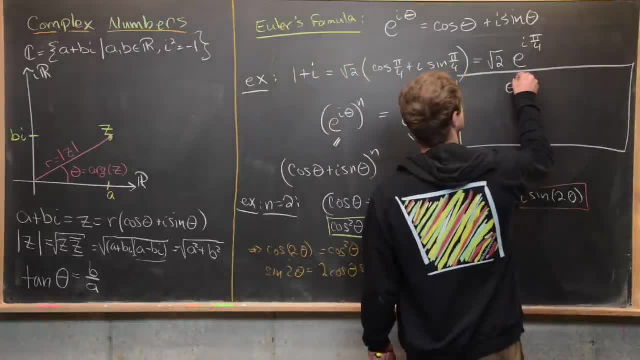 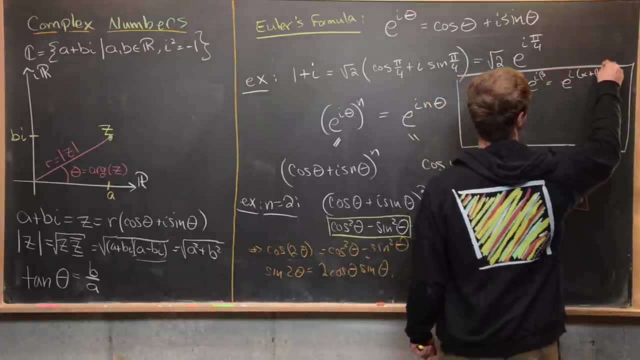 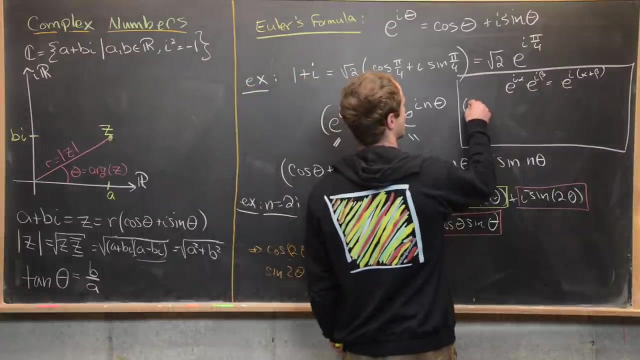 different ways. So we can expand e to the i alpha times, e to the i beta. So on the one hand that's e to the i alpha plus beta, And then on the other hand we can expand this using Euler's formula. So over here on the left we have cosine alpha plus i sine alpha. 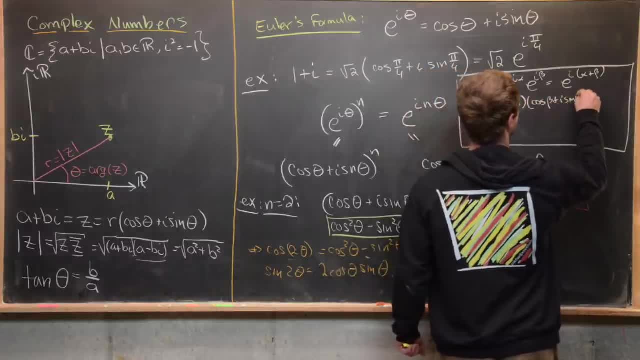 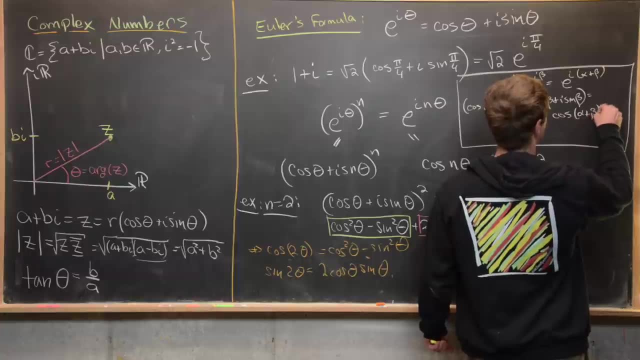 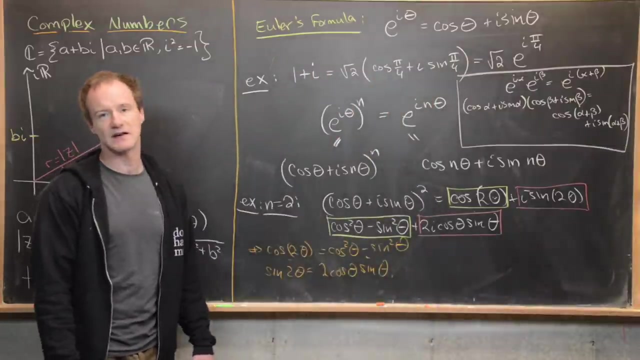 Times, cosine beta plus i sine beta. And then over there on the right we're going to have cos alpha plus beta plus i sine alpha plus beta. Now we can expand the left hand side of that equation, extract real and imaginary parts and compare it to the right hand side of the equation. 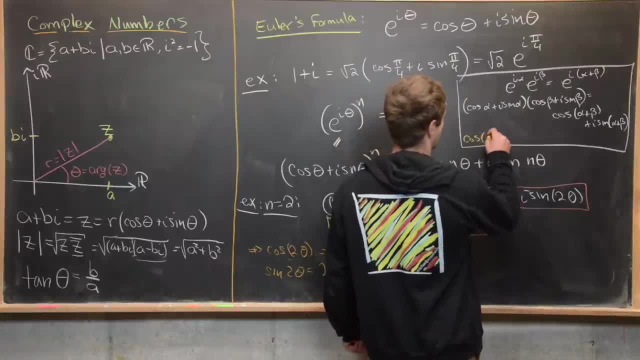 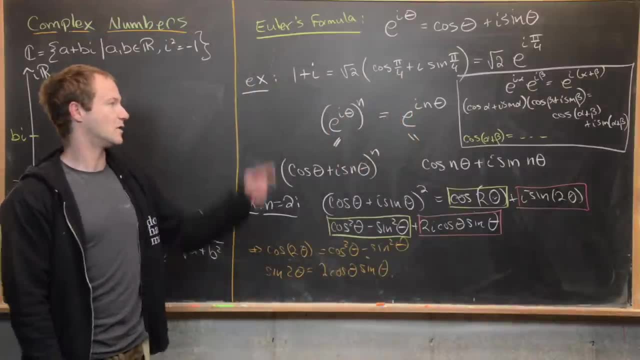 and come very quickly up with some formulas like cosine, alpha plus beta equals some stuff. I'll let you guys check what exactly you get by multiplying out that left hand side of the equation. Okay, So now let's go ahead and clean this up and we'll look at some nice examples. 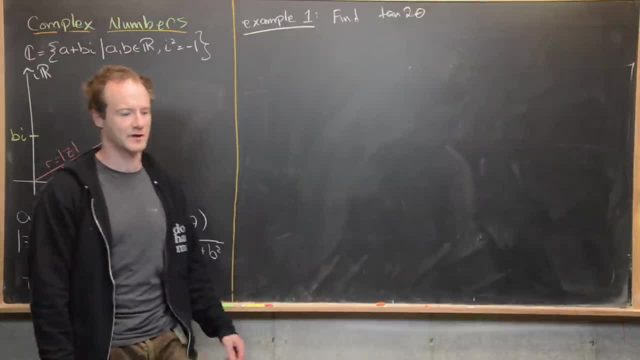 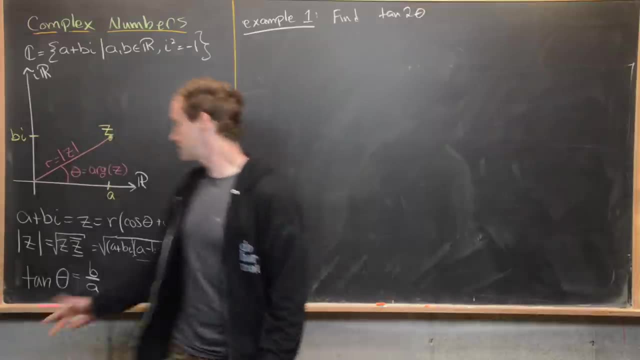 Okay, For our first example, we're going to calculate a double angle formula for tangent And, even though we just looked at Euler's formula, we're going to do this a slightly different way, just being motivated by the geometry of the polar form of a complex number. 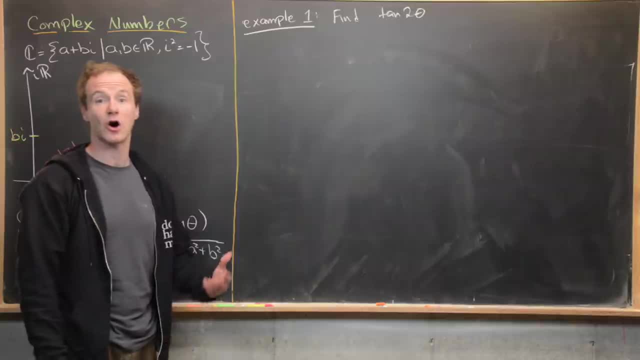 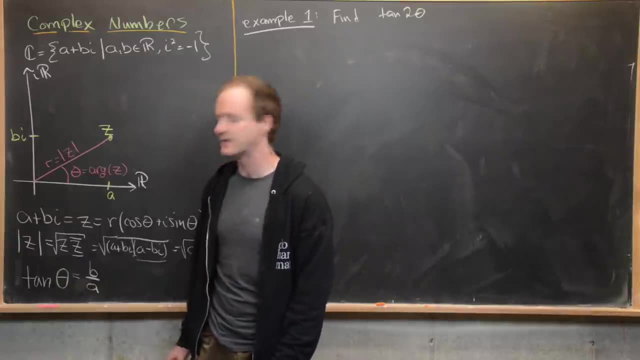 But now we're going to want to find the simplest complex number, whose argument is theta, And we can do that via looking at this formula down here. So we know, tangent of theta, in other words tangent of the argument, is equal to b over a. So we might as: 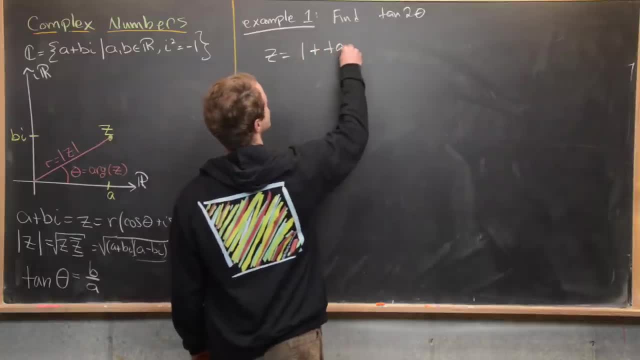 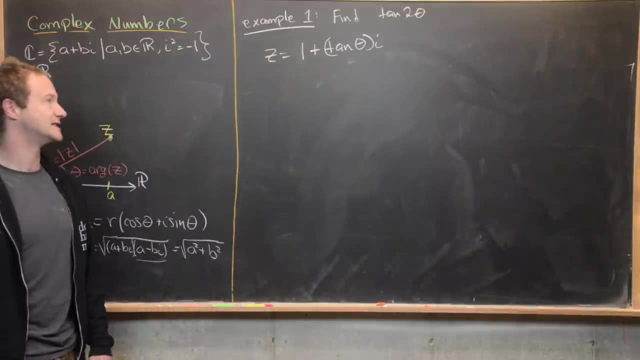 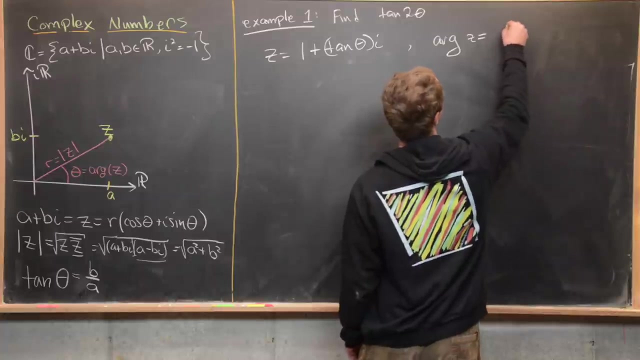 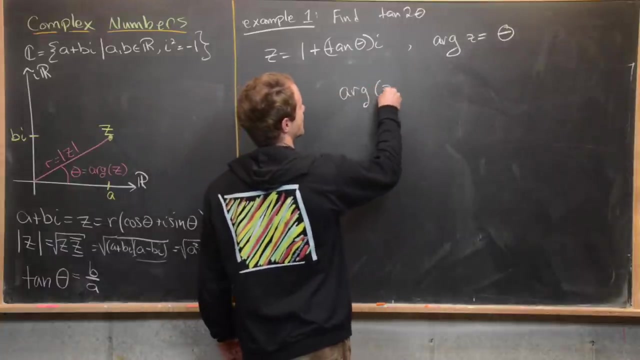 well set z equal to one plus tangent theta times i. In other words, a is being played by one and b is being played by tangent of theta. But now, under this setup, we can say that the argument of z is equal to theta Great, But now we can jump from there to say that the argument of z squared. 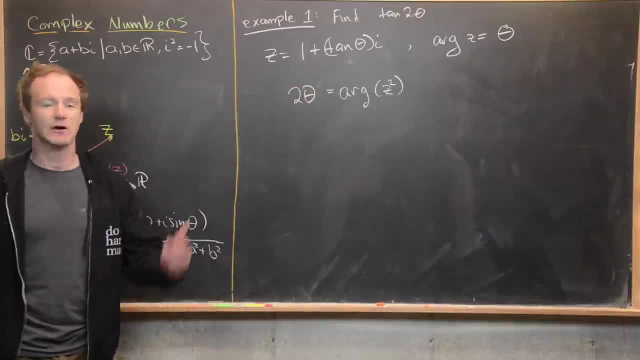 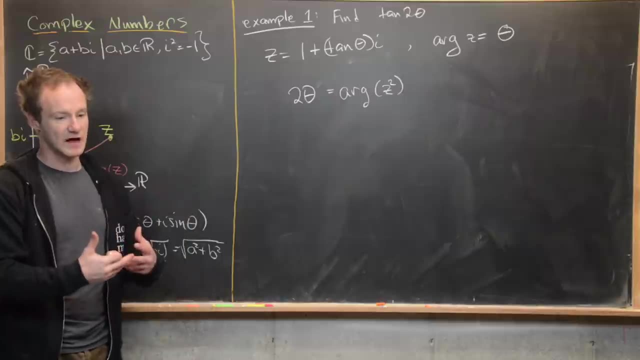 is going to be equal to two theta, Because that's how arguments work. Just think about the Euler's formula with e to the i alpha and e to the i beta. If you multiply those two numbers, you add the angles or you add the arguments. So if you square a complex number, you're going to add its argument. 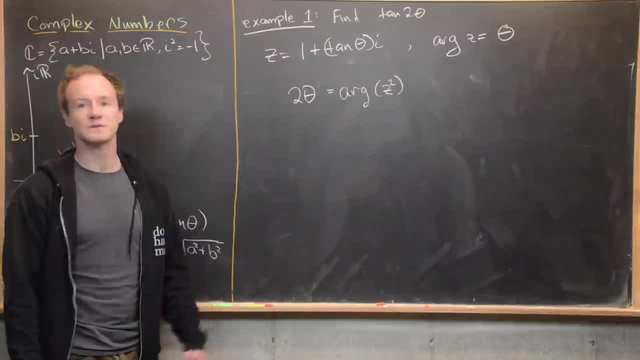 with itself. It's like, for example, if you're going to add a complex number, you're going to add a complex number. So if you're going to add a complex number, you're going to add a complex number from that rotation principle. But now I want to flush out this z squared object a little bit. So 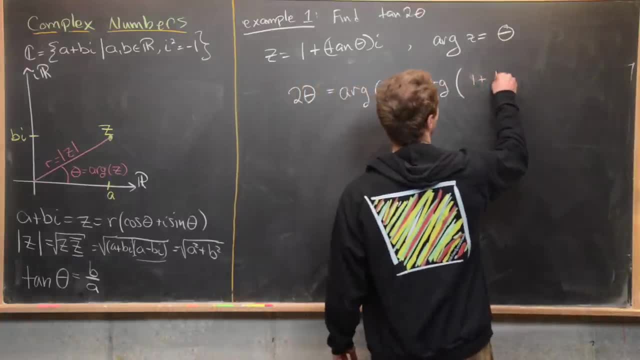 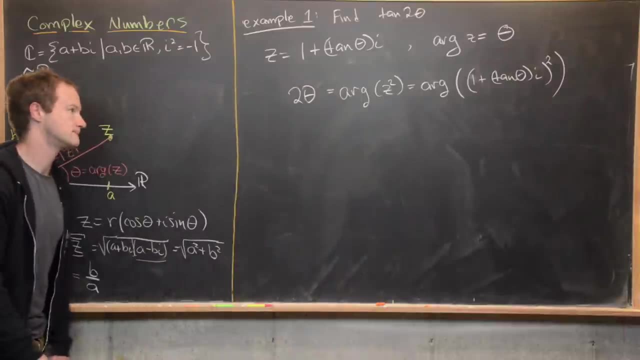 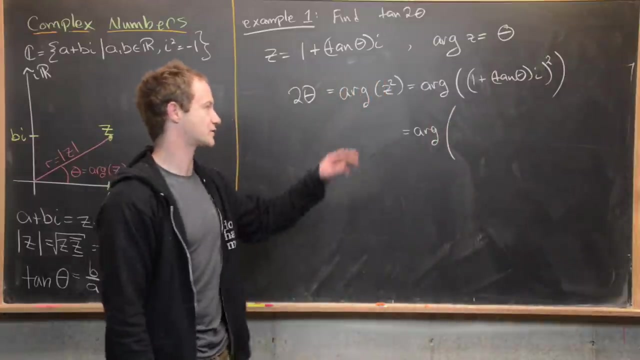 here we have the argument of one plus tangent theta times i quantity squared, like that Good. But if we calculate that, we have the argument of now. if we multiply out this right hand side, we'll get one minus tangent squared theta. So that's. 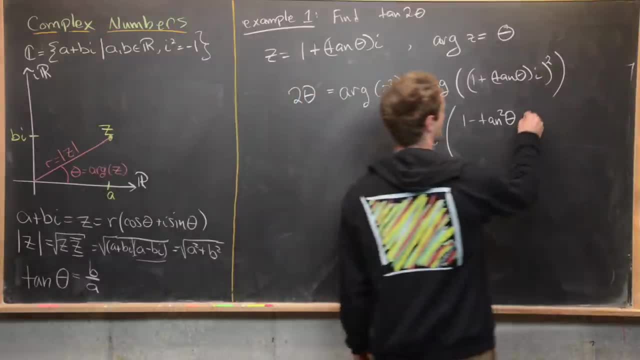 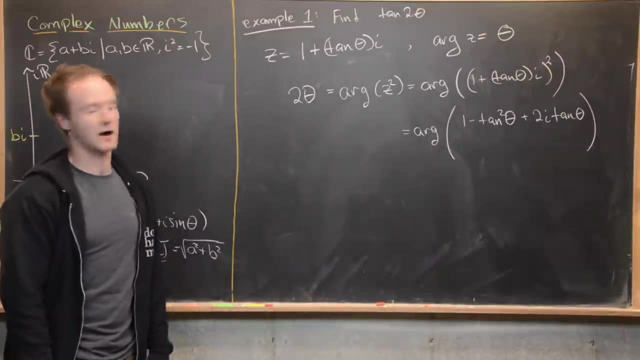 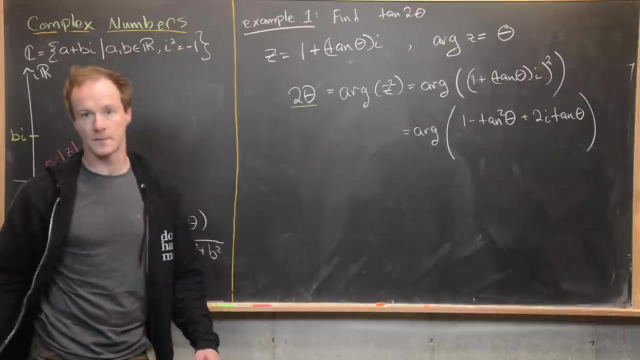 we get for the real part And for the imaginary part we'll have plus two times- i times tangent theta like this. So we have the argument of that complex number. So just to reiterate what we have going on here is two theta equals the argument of this complex number, which has real part. that 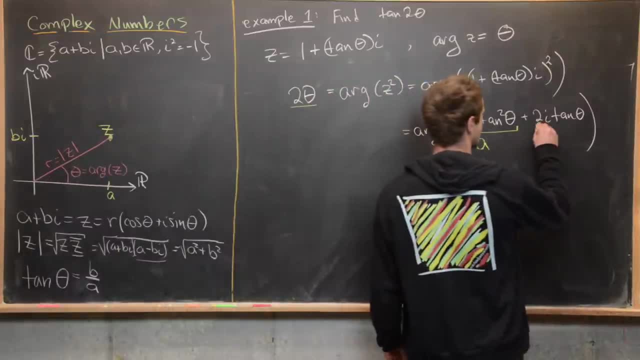 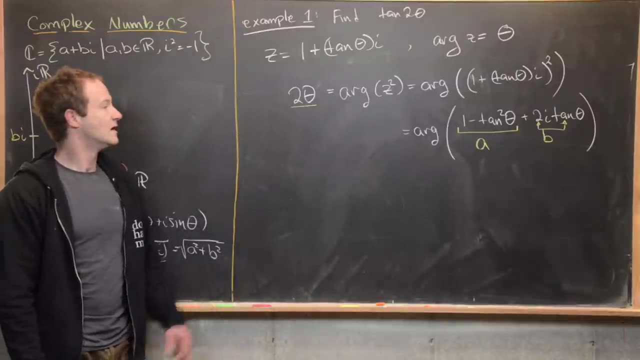 which I'll call a, and it has imaginary part this two times tangent theta. So I'll call that d theta And I'll call that b. Good, But now we're going to use the fact that tangent of the argument is equal to b over a, And that follows from this, just where theta has been replaced with two theta or 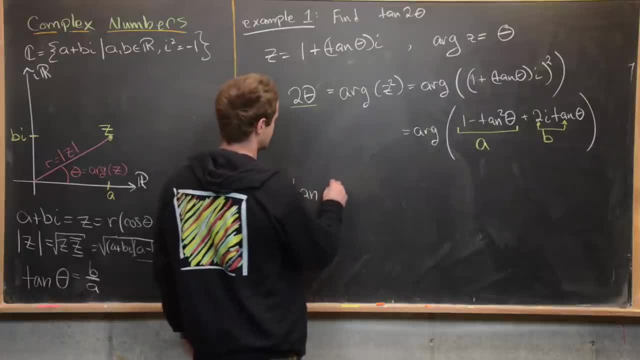 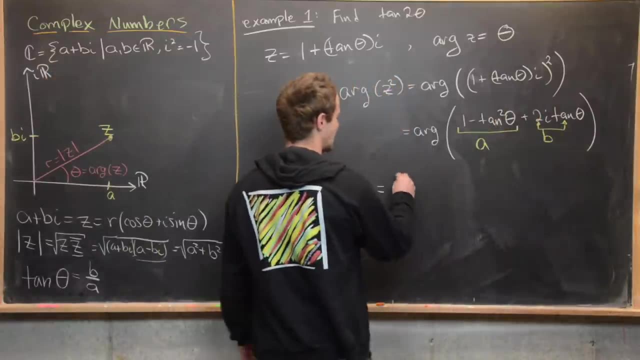 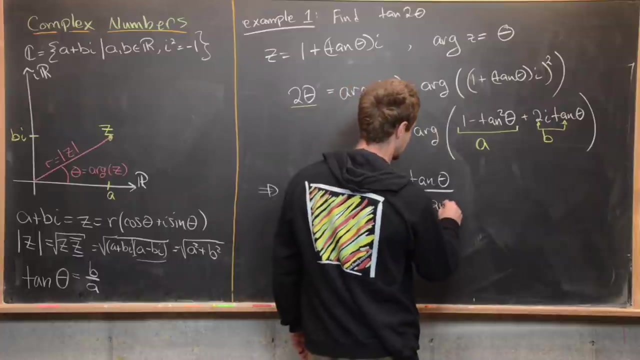 something. So let's take the tangent of both sides. So tangent of two theta, that's tangent of the left hand side, equals the imaginary part divided by the real part. So that leaves us with tangent of theta times two over one, minus tangent squared of theta, And that derives a semi familiar double. 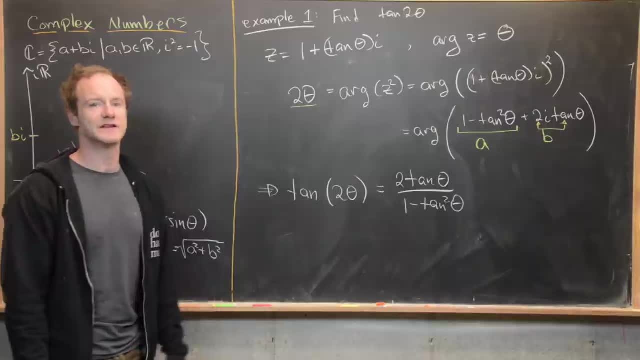 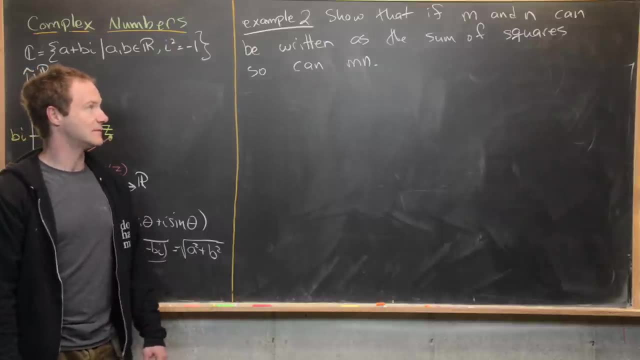 angle formula for tangent. Okay, so let's go ahead and get rid of this And we're going to look at another example. Okay, for our next example, we're going to show that if m and n, which are natural numbers, can be written as the sum of squares, so can m times n. 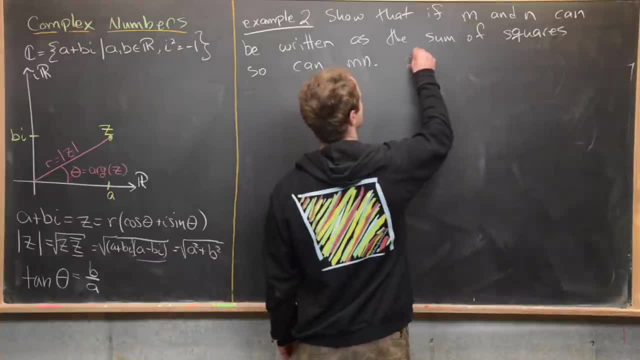 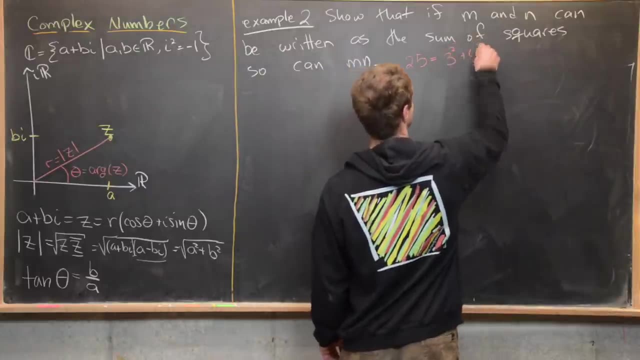 So let's just like look, for example, we know the number 25 can be written as the sum of squares, because it's equal to three squared plus four squared. Well, that's just part of a Pythagorean triple, But it turns out that there are lots of numbers that can be written of sums. 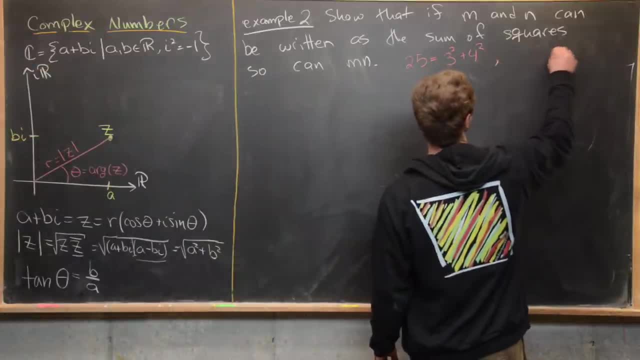 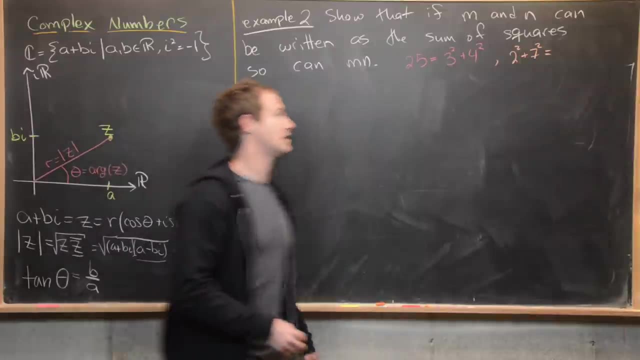 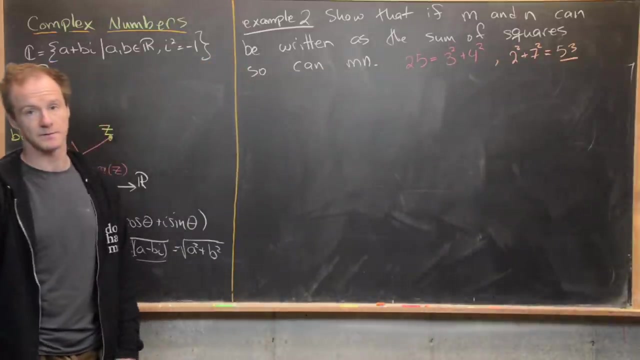 of squares that are not Pythagorean triples. Like, for instance, if we take two squared plus seven squared, so that's going to be 49 plus four, So that's going to be 53.. So 53 is one of these numbers that can be written as a sum of squares. 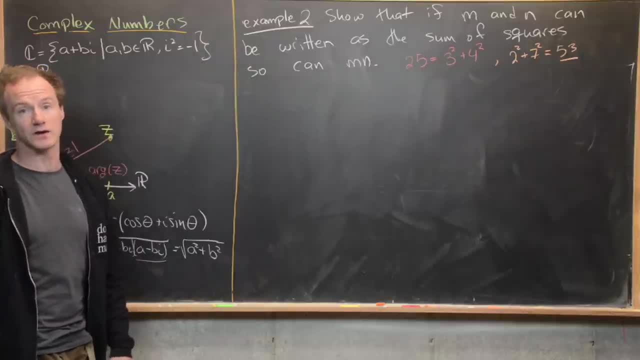 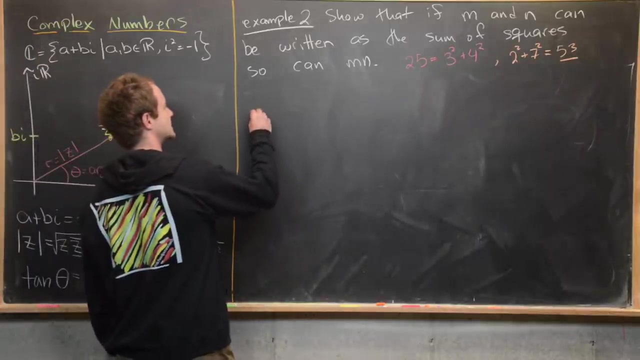 here. this is saying that the set of the sum of squares is closed under multiplication. That is, if you've got one and you've got another one, you multiply it. you've got a new number that can be expressed as a sum of squares. Okay, good, So maybe let's get to it. So how do you do this? 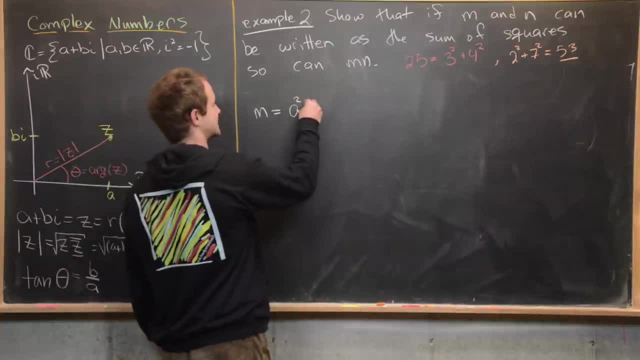 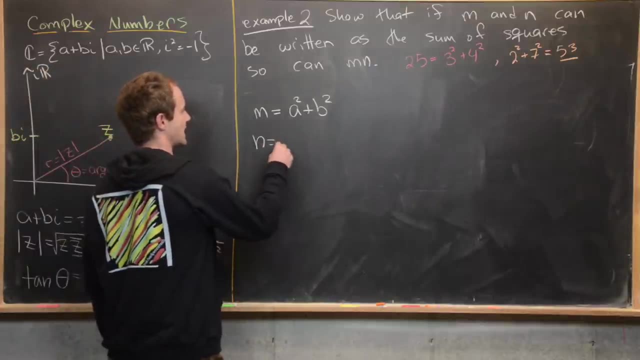 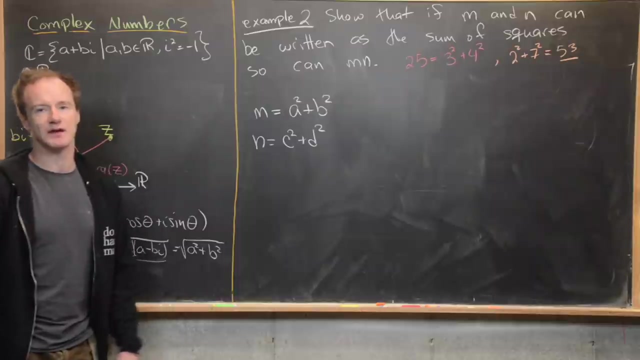 So you're going to take m and you're going to write it as its sum of squares, a squared plus b squared, where those are all natural numbers. Then we'll do the same thing for n. That's going to be equal to c squared plus d squared. So, using integers, these expressions are not immediately. 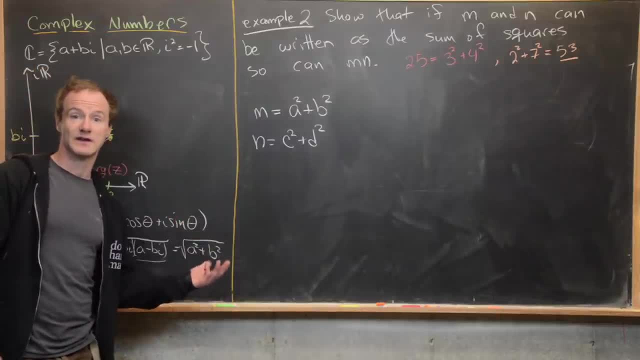 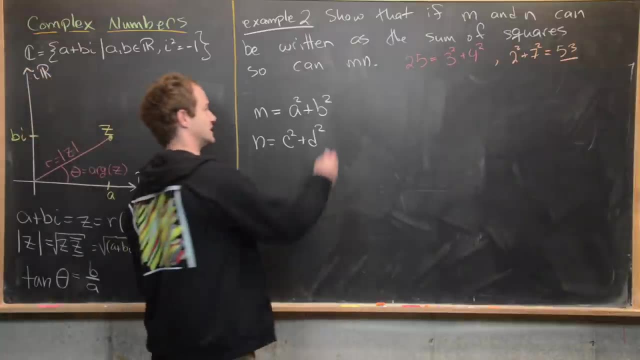 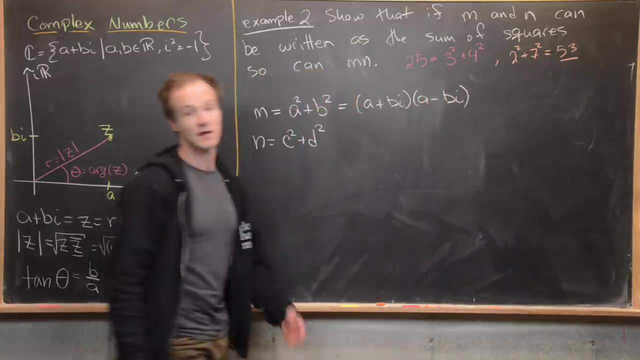 factorable. But if we include the complex number i along with the integers, sometimes called the Gaussian integers, we can immediately factor these. Notice, this first one is going to factor like a plus bi times a minus bi, like we've seen. And then the second one is going to factor like: 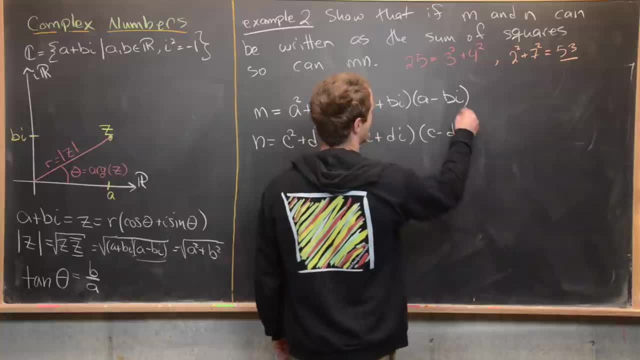 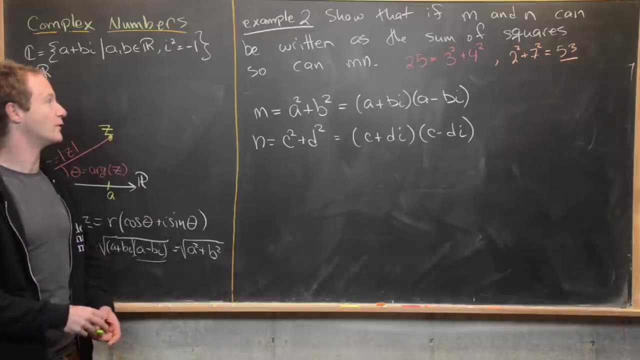 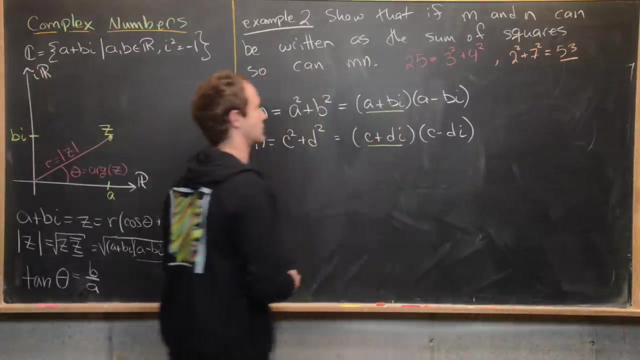 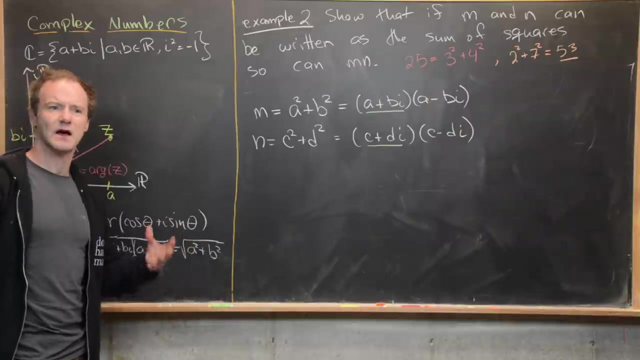 c plus di times c minus di. Good, And this factorization has the seeds of exactly what we want: to express m times n as a sum of squares. For instance, if I take this number right here and this number right here- a plus bi and c plus di- and I multiply those, that's going to be a big tool. 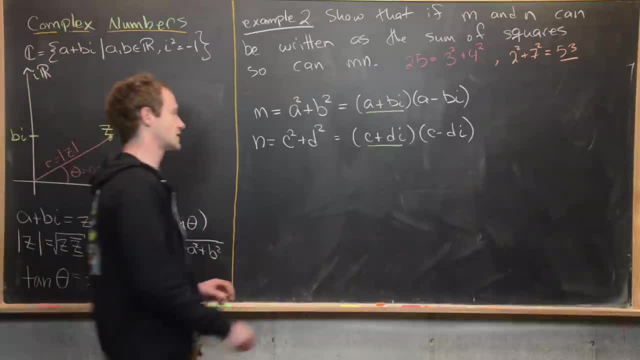 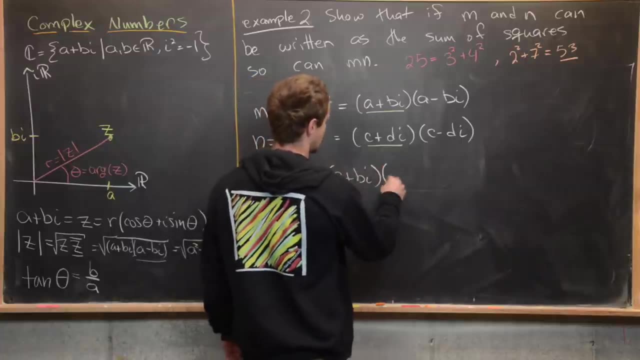 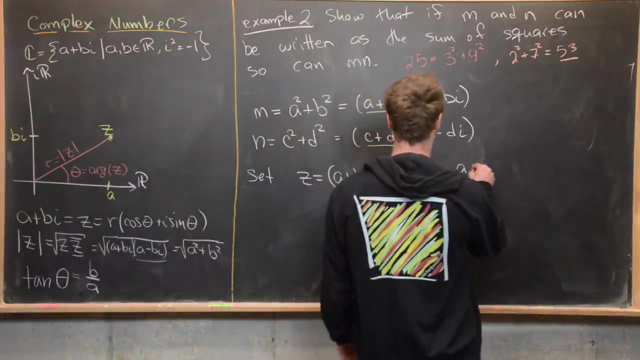 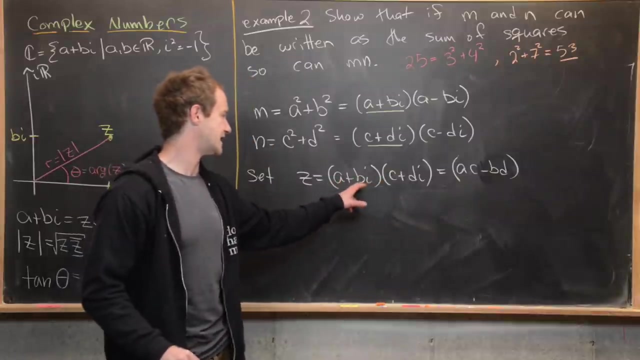 for writing m times n as the sum of squares. Okay, so let's go ahead and do this. So let's set a plus bi equal to a plus bi times c plus di, And then notice that we can multiply this out. This is going to be ac plus- sorry, minus bd. Again, that would be the a times c and the bi times di. 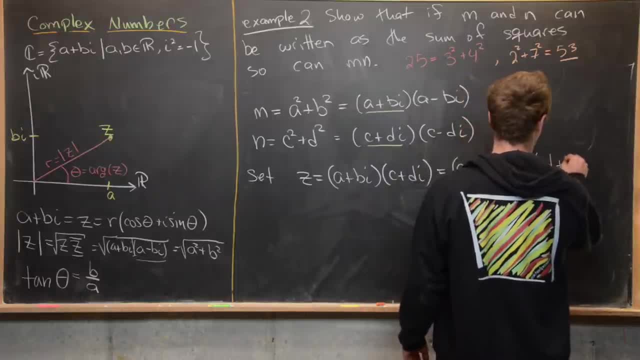 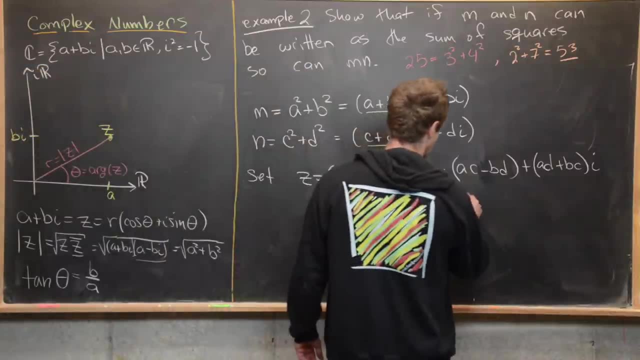 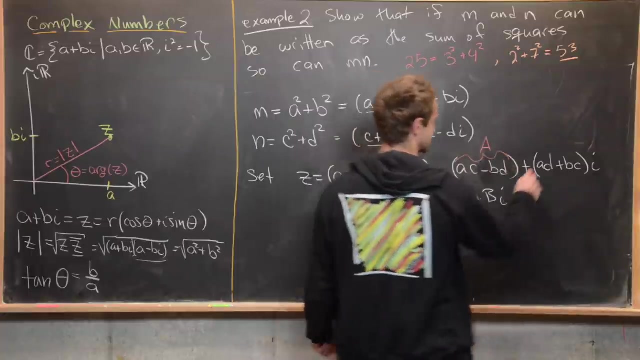 And the next we're going to have plus ad plus bc times i like that. Now I want to go ahead and write that as capital A plus capital B times i, where I just absorb all of these numbers into capital A and all of those numbers into capital, And those are still integers, because 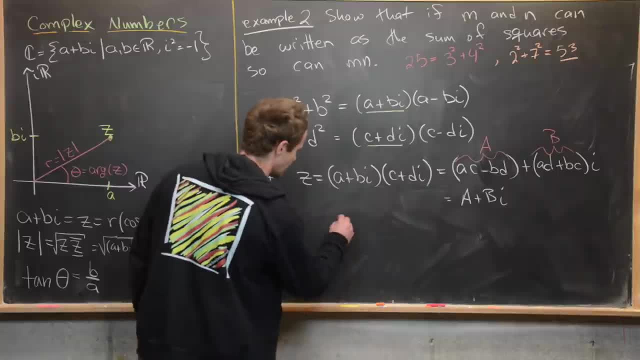 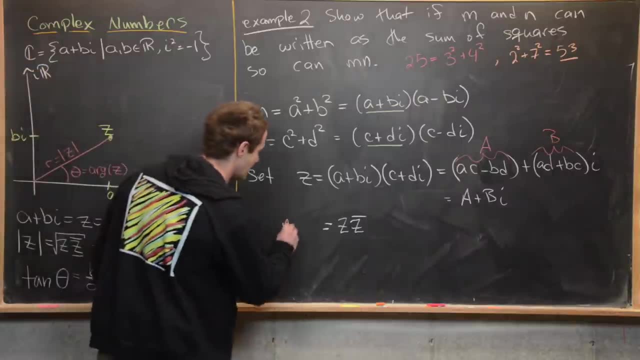 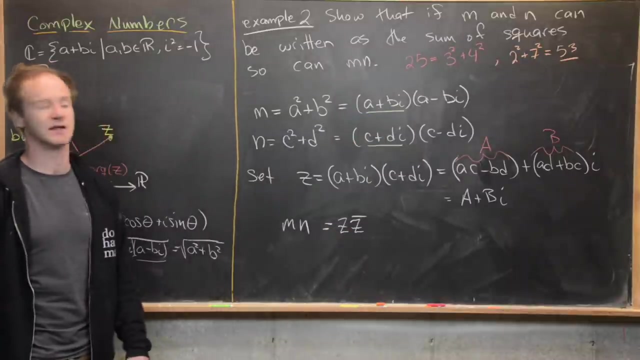 they're combinations of integers. Now the next thing that I want to notice is, if I take z times z bar, on the one hand I'm going to get m times n, because z times z bar is just the multiplication of this line times this line. 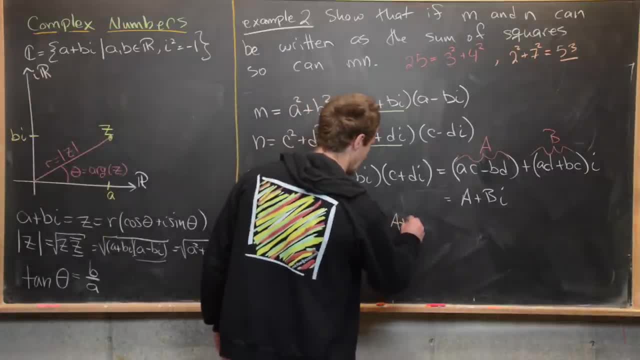 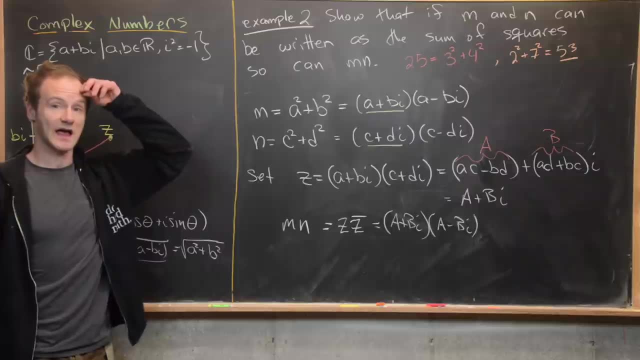 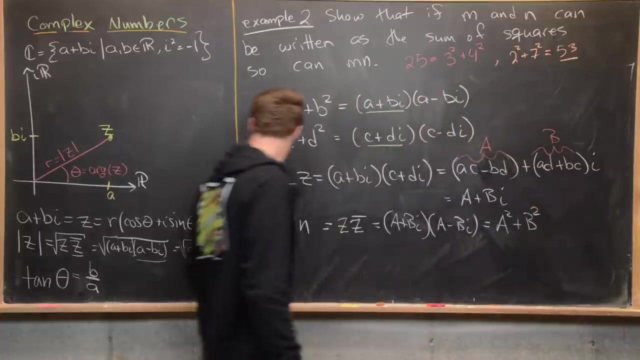 But then, on the other hand, it's going to be equal to a plus bi, where I have capitals, and capital A minus bi, where capital A and B are defined like that. But this is equal to capital A squared plus capital B squared. So I have exhibited the product of m and n. 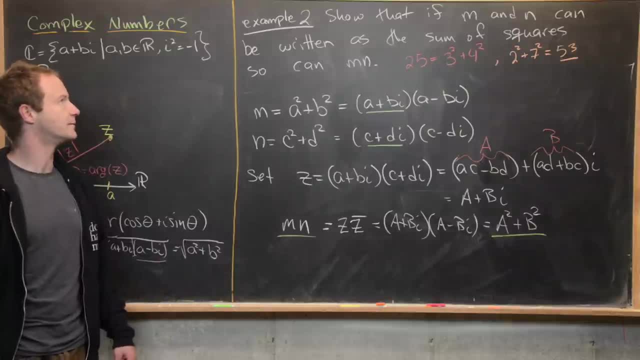 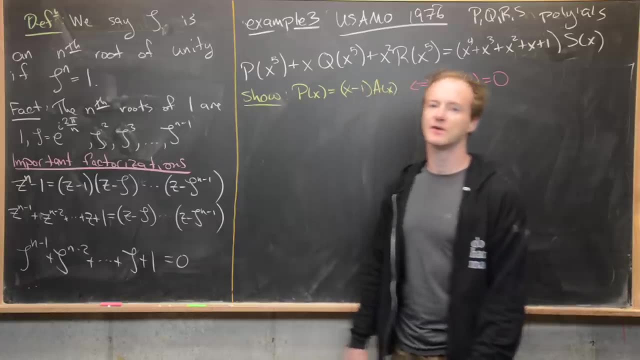 as the sum of two squares, which is exactly what we wanted to do. Okay, so I'll clean this up. Then we're going to look at the notion of roots of unity before our last example. So we're going to finish this video off with: 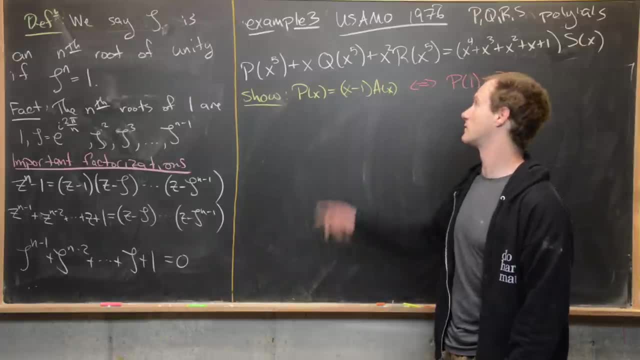 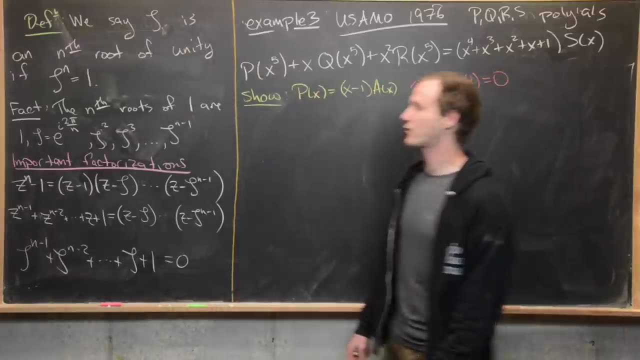 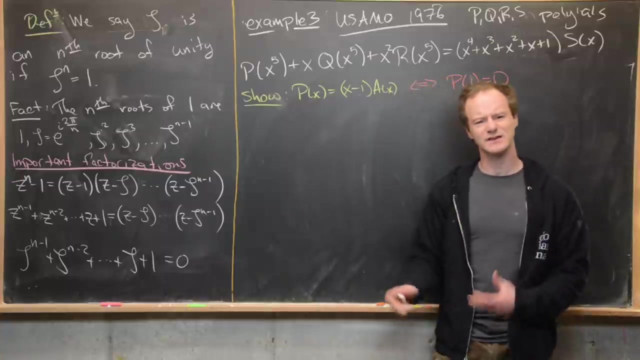 the notion of the nth roots of unity as well as a problem from the USA National Math Olympiad. Okay, so we say that zeta is an nth root of unity if it satisfies the equation: zeta to the nth power equals one. So these are like the nth roots of the number one. And here's 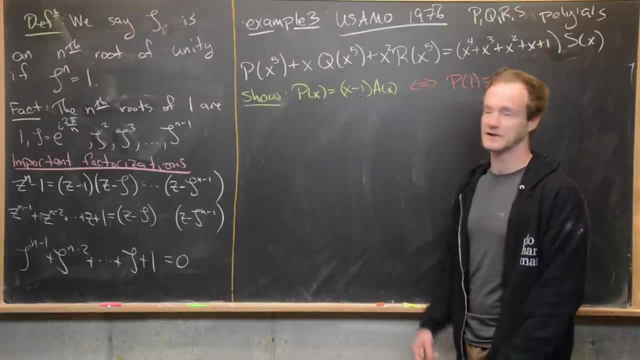 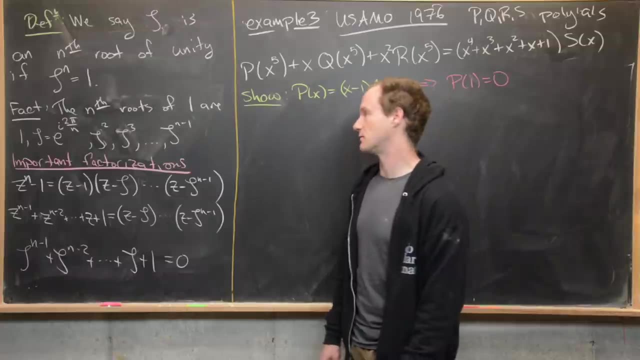 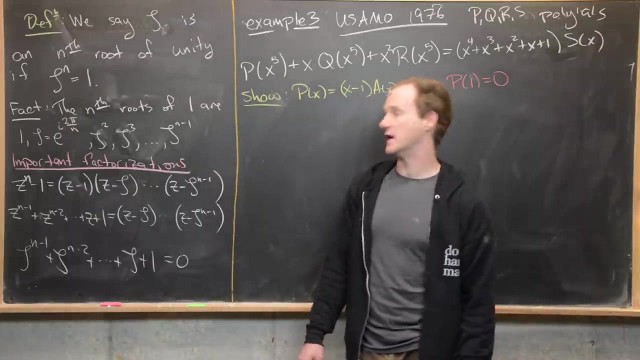 a fact, and so we're not going to prove this, but you could grab a proof for this pretty easily. So what we're going to do is: the nth roots of unity are these following n complex numbers, And so there's one, and then there's zeta, which is equal to e, to the i, 2 pi over n. 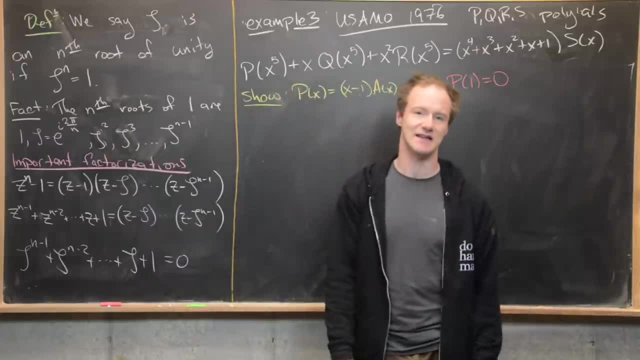 And then there's zeta squared, zeta cubed, all the way up to zeta, to the n minus one, where what I'm doing is I'm squaring this complex number e to the i 2 pi over n cubing. 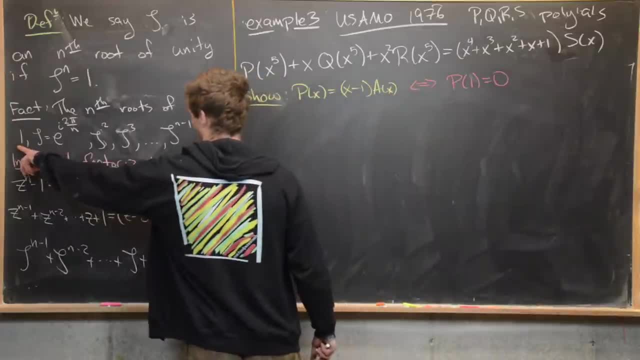 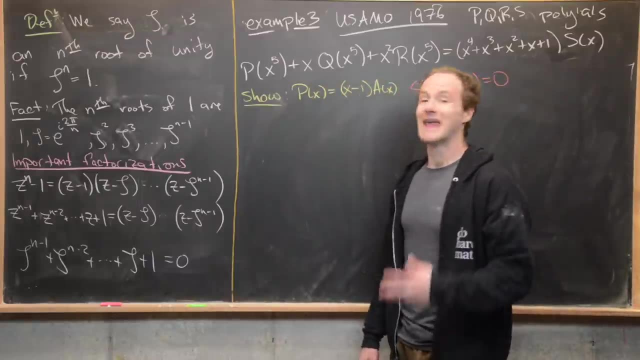 it, and so on and so forth. So notice, I've got the zeroth power of zeta, the first, the second, the third, I've got all the way up to the n, minus first, And those are the n total different nth roots. 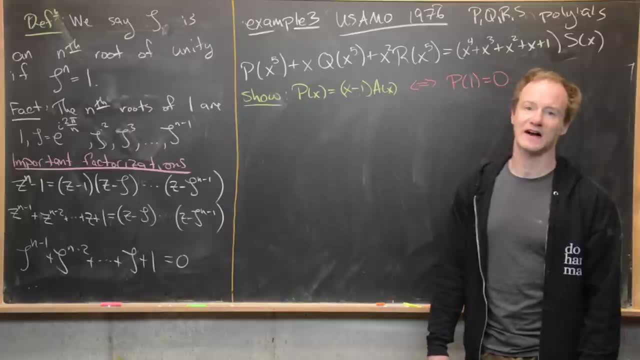 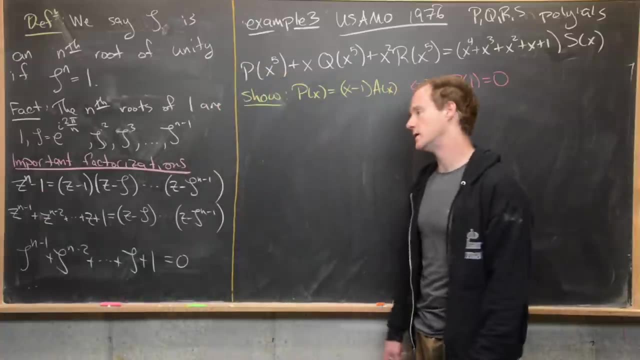 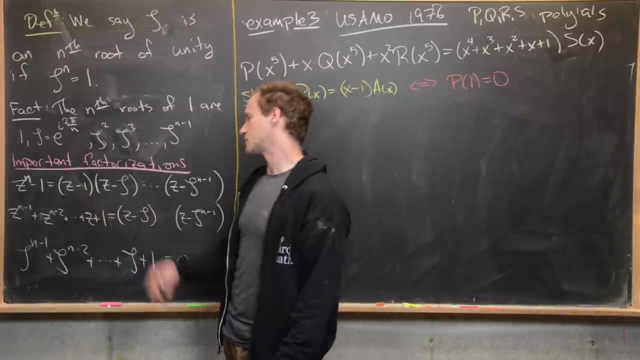 of unity. Okay, and then a really important factorization involving these nth roots of unity goes like this: So we've got z to the n minus one factors as a product of z minus each of these roots of unity. So we've got z minus one times z minus zeta, times z minus zeta, squared all. 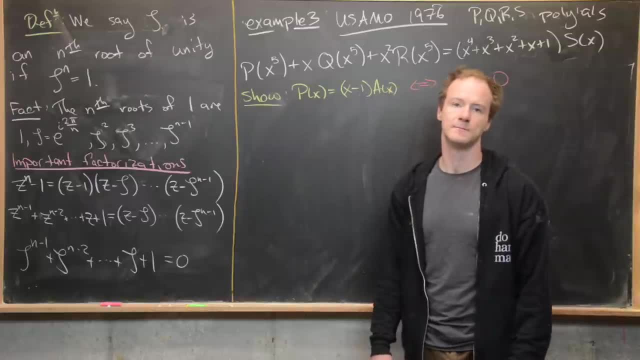 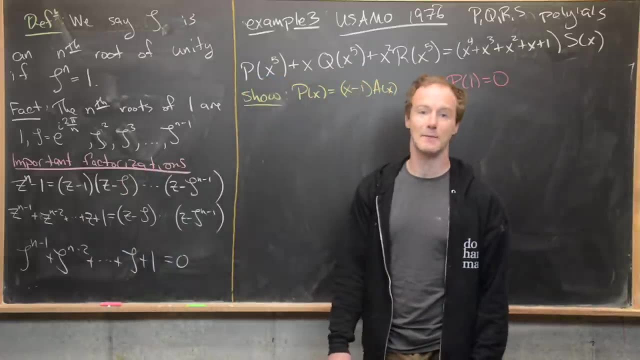 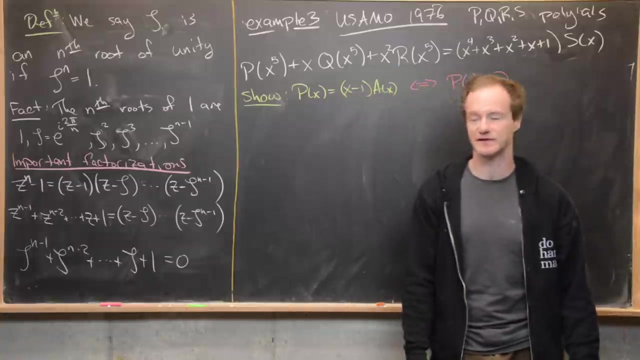 the way up to z minus one. Now, if we go ahead and take both sides of this equation and divide it by z minus one, well, the right hand side is going to look essentially the same, just without a z minus one as part of this product, but the left hand side is going to simplify to this object. 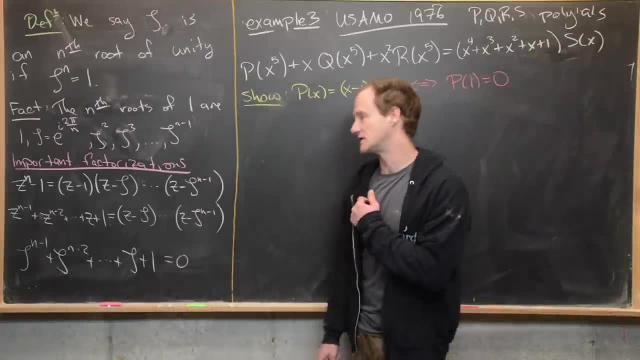 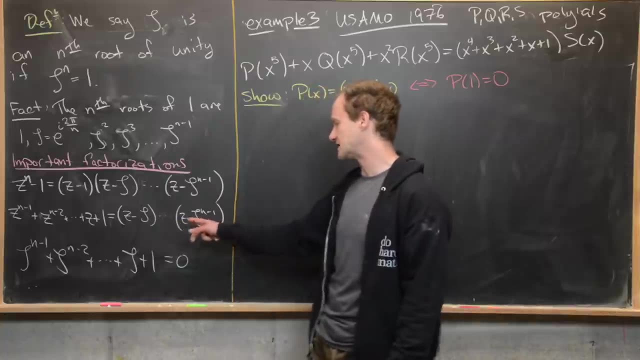 And this is an important formula. So z to the n minus one times z to the plus, z to the n minus two, all the way down. Okay, plus 1 is z minus zeta times z minus zeta, squared all the way up to z minus zeta, to the n minus 1.. 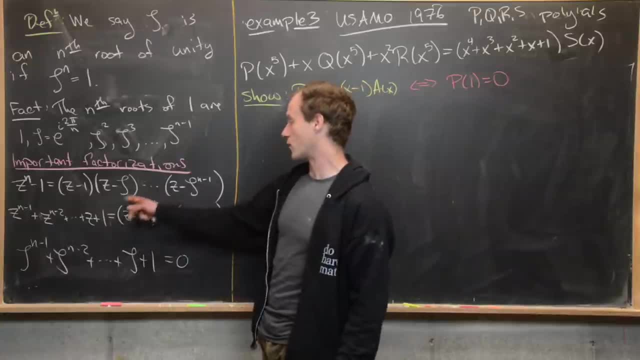 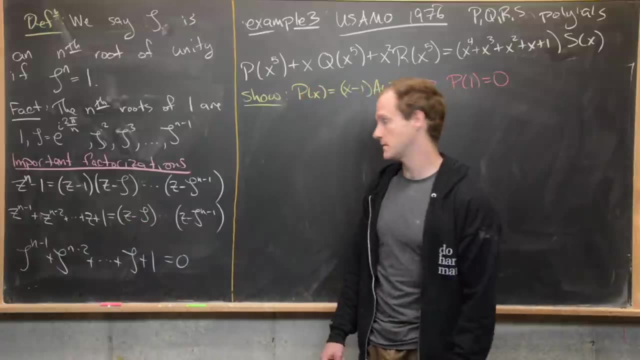 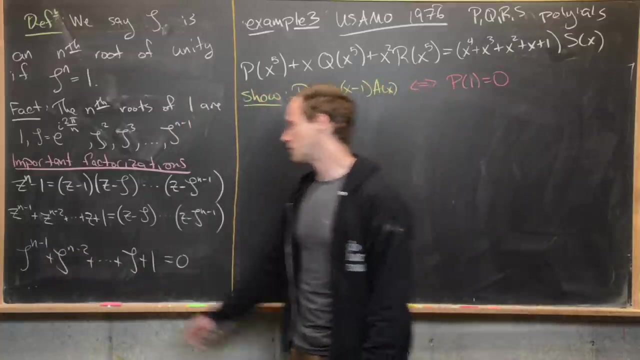 Okay, but now if we evaluate the right hand side of this equation at zeta, notice, this first one is zeta minus zeta, which is 0, and then the left hand side of the equation will be this sum of the all the roots of unity. So notice, we have zeta to the n minus 1 plus zeta to the n minus 2, all the way. 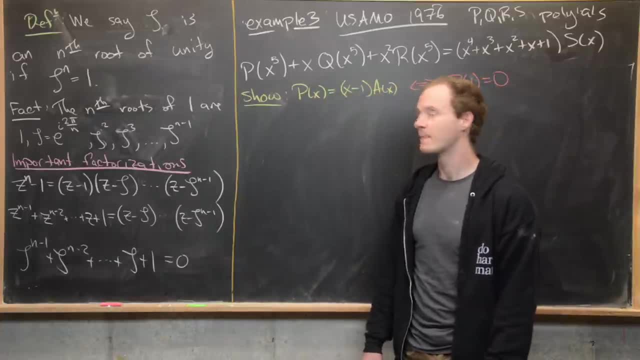 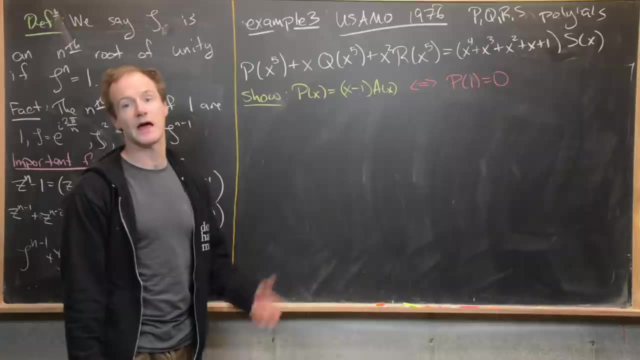 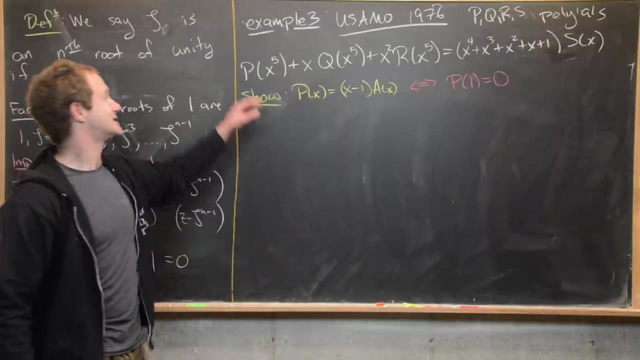 down, plus zeta, plus 1, that equals 0.. Okay, so for our example, we want to look at, like I said, this problem from the USA, Math Olympiad 1976, and we want to have polynomials p, q, r and s that satisfy the following equation. So we've got p evaluated at x to the fifth. 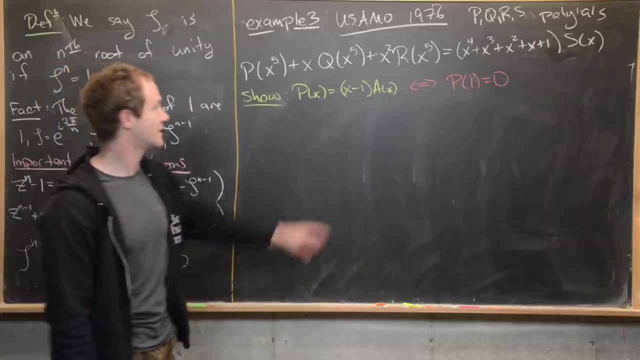 we've got zeta to the n minus 1, plus zeta to the n minus 2, all the way down, plus zeta plus 1, plus x times q, evaluated at x to the fifth, plus x squared times r, evaluated at x to the fifth. 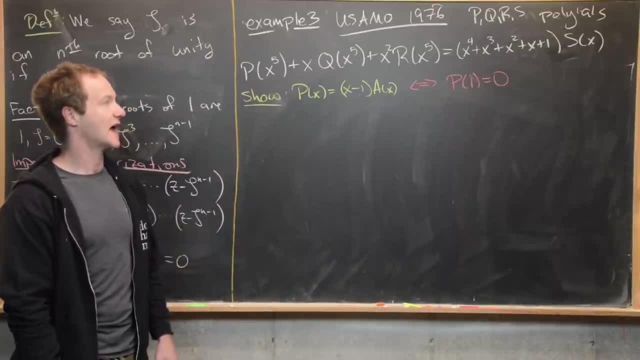 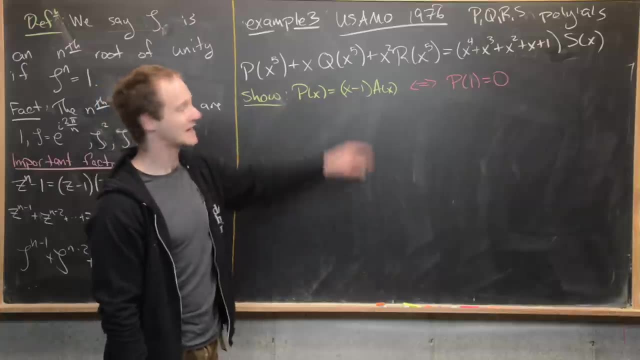 equals x to the fourth, plus x cubed, plus x squared, plus x plus 1.. And what we want to show is that x minus 1 is a factor of p of x. In other words, p of x can be written as x minus 1 times a. 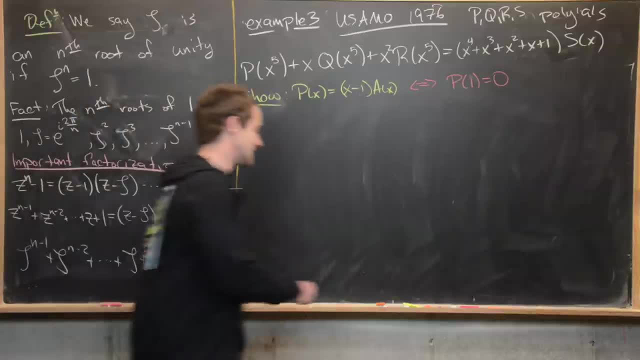 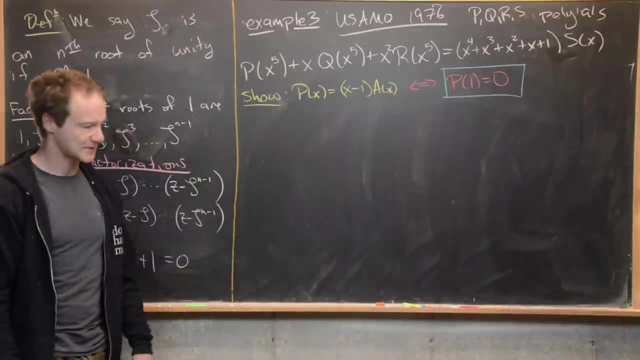 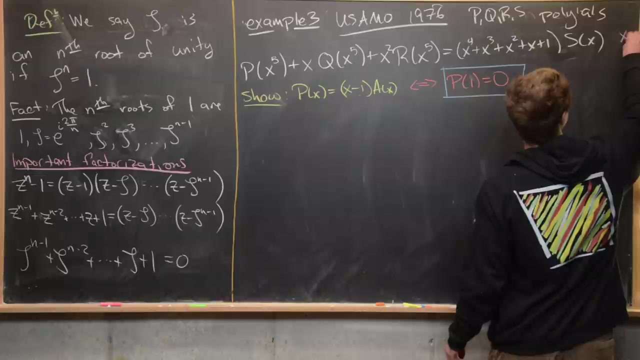 of x, where a of x is another polynomial. But that is equivalent to the following statement: that p evaluated at one is zero. And that's exactly what we're going to show: that p evaluated at one is zero. So how we're going to do this is we're going to take this starred equation. 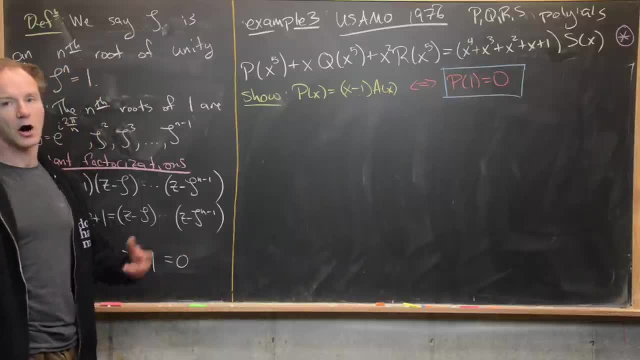 and we're going to evaluate this starred equation at all- of the roots of unity. and which roots of unity? Well, the fifth roots of unity, because, notice, we've got an x to the fifth here. So any fifth root of unity to the fifth power is going to be one. And then 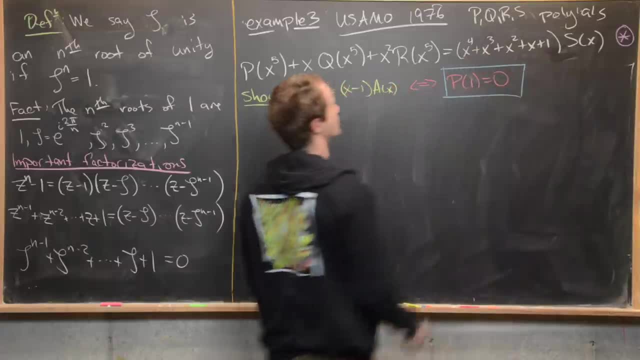 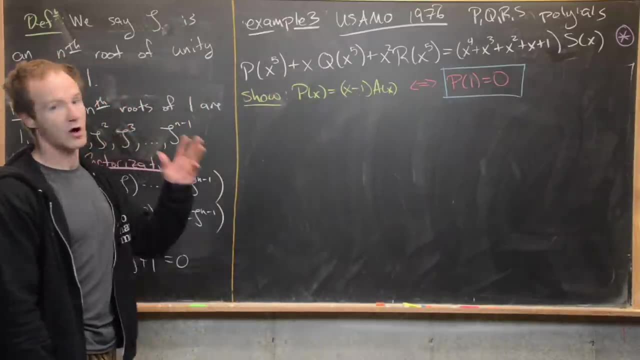 Any fifth root of the unity put into this polynomial right here is going to be equal to zero by this observation down here. Okay, so let's maybe look at all five equations. So let's say we have x equals 1. That's our first equation. 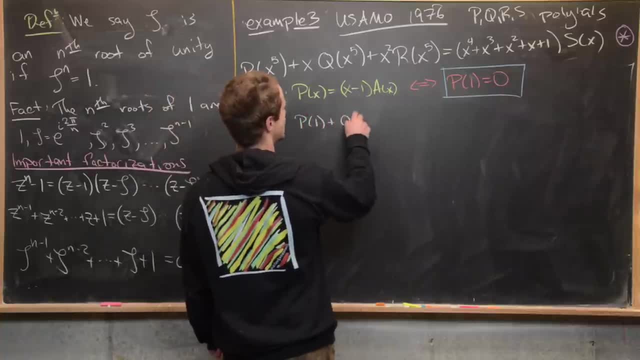 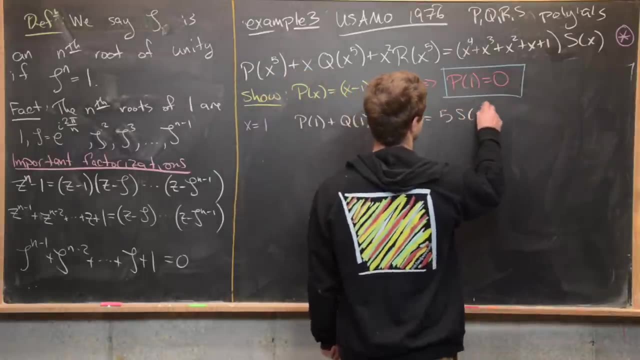 So notice that's going to give us p of 1 plus q of 1 plus r of 1 equals, So that's going to be 5 times s of 1.. So in fact this is not super helpful and we don't even really need this one. 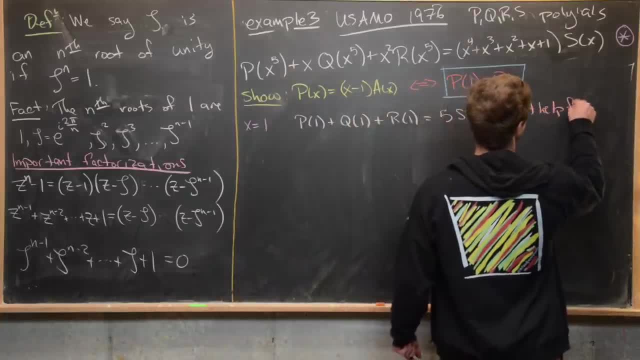 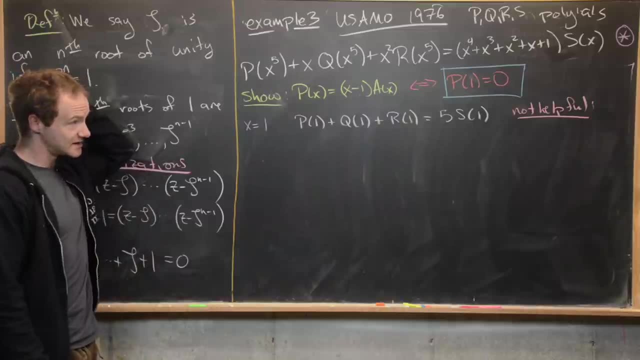 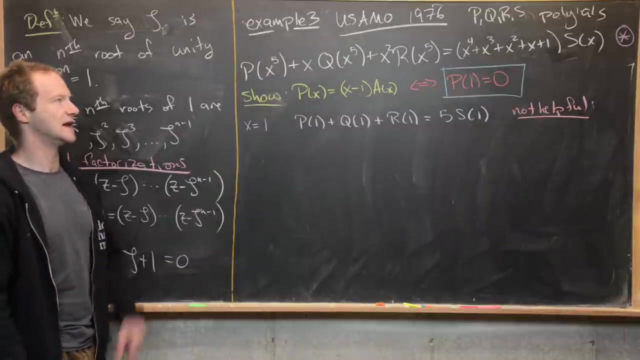 So this is not helpful. I mean, maybe it was useful to look at it, but it's not helpful for finding our solution here, because it doesn't allow us to get rid of anything. But now notice, if we look at the other fifth roots of unity, so the ones that are not equal to 1,- 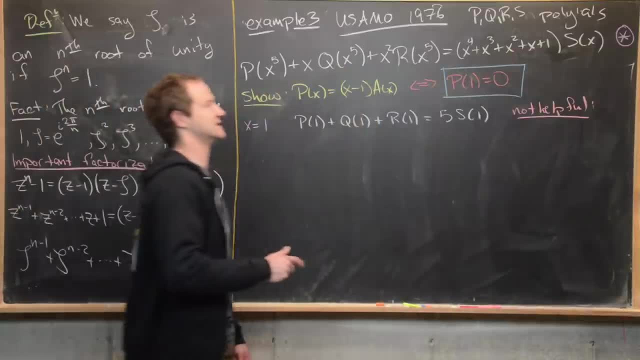 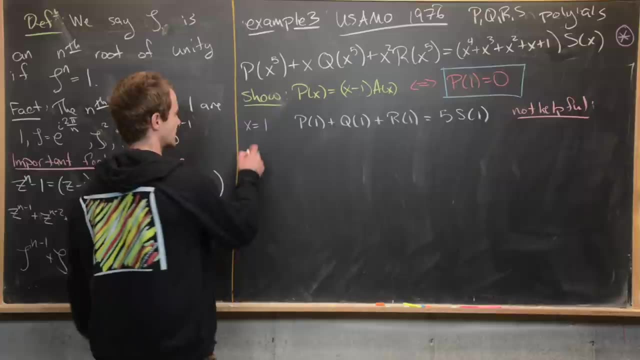 those are the ones that equal zero when we plug them into this x to the fourth, plus x cubed, plus x squared, Plus x plus 1 object. So that's what we want to look at. So here let's go ahead and set zeta equal to e to the i 2 pi over 5.. 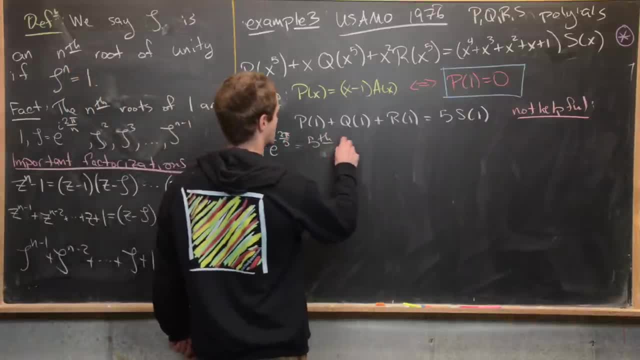 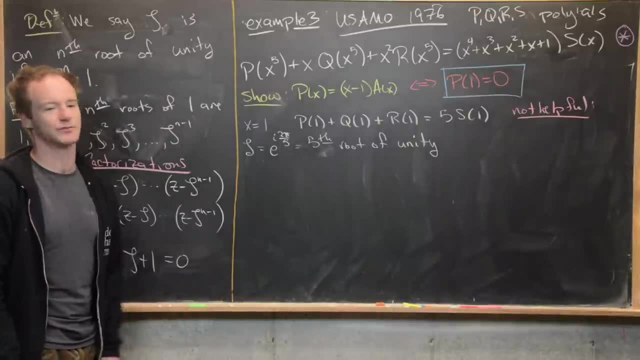 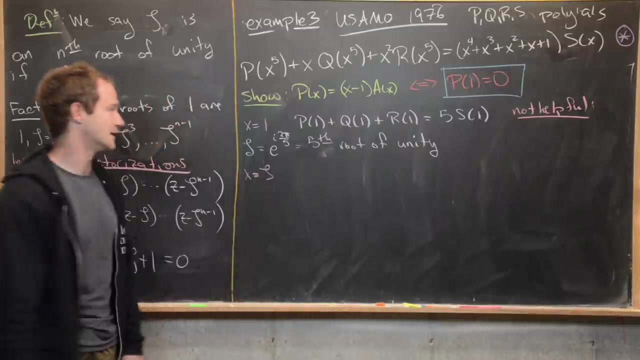 So, in other words, this is a fifth root of unity. Sometimes we would say a primitive fifth root of unity, but since 5 is a prime number, that doesn't really make a difference. Okay, so let's go ahead and look at the case when x is equal to zeta. 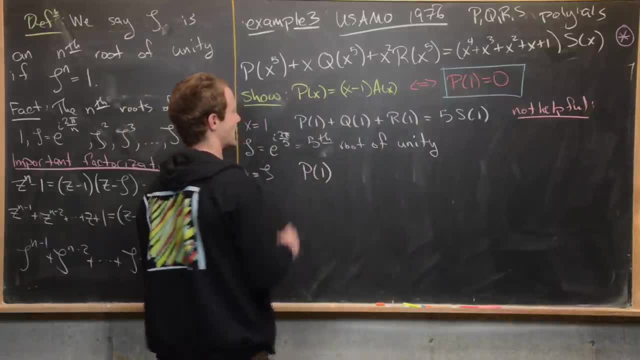 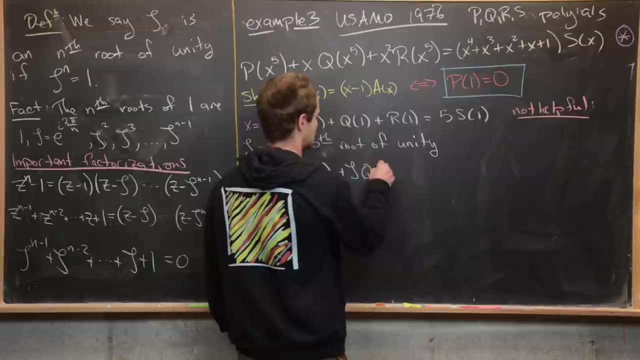 So This equation is going to turn into p evaluated at 1, because zeta to the fifth is 1, given that it's a fifth root of unity, plus zeta q of 1, plus zeta squared r of 1 equals 0.. 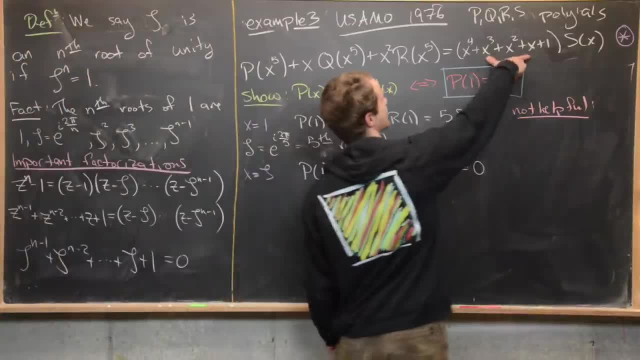 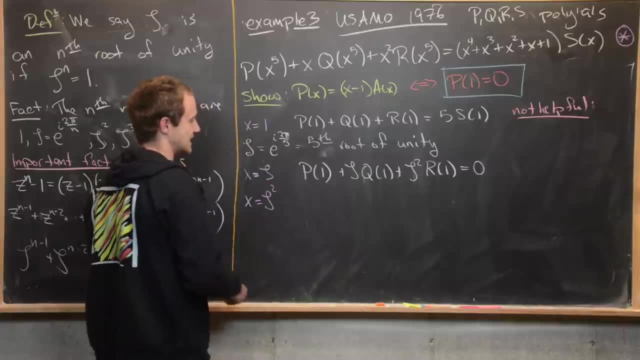 We know it's equal to 0 because again, when we plug that into this thing right here, we get 0 by our earlier discussion. Now let's look at the other cases. So x equals zeta squared, So that's going to give us p of 1 again. 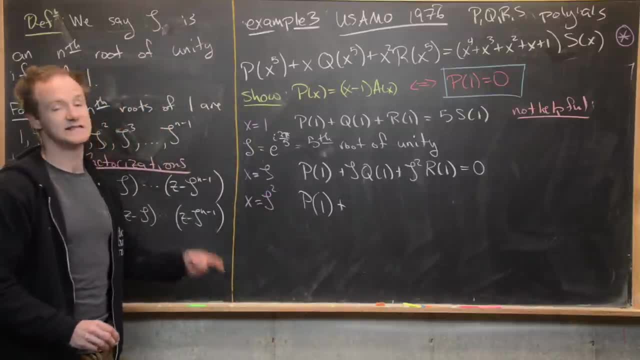 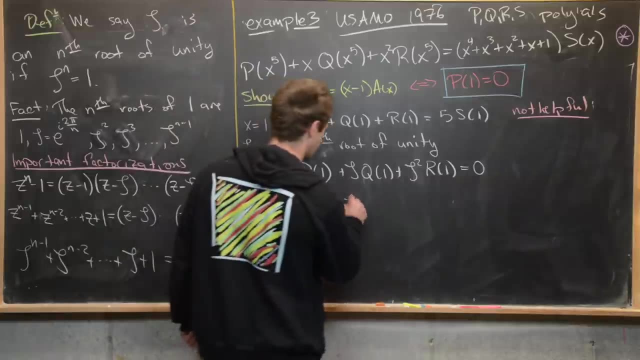 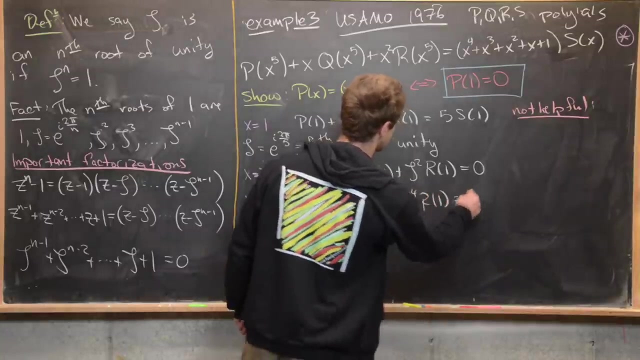 So, again, if we evaluate this zeta squared, we're going to get zeta to the 10th, but that's zeta to the fifth squared, but that's 1 squared. So we're good to go there. Now we have zeta squared, q of 1 plus zeta to the fourth. r of 1 equals 0.. 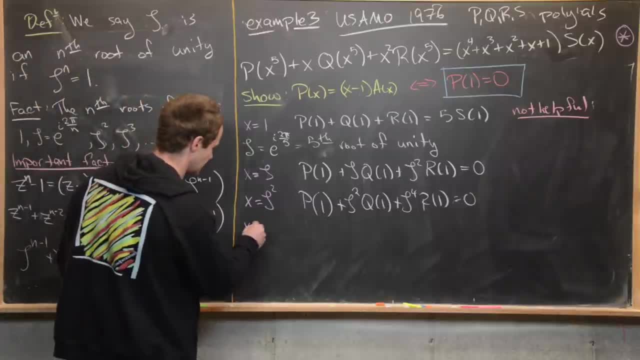 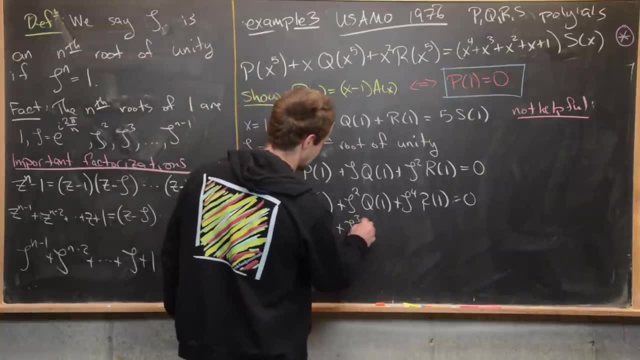 So that's what we get for the zeta squared. Let's look at the zeta cubed. So here we're going to get x equals zeta cubed. So again we'll have p of 1 plus zeta cubed q. 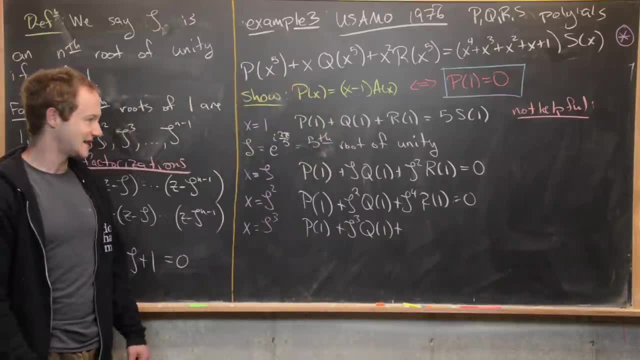 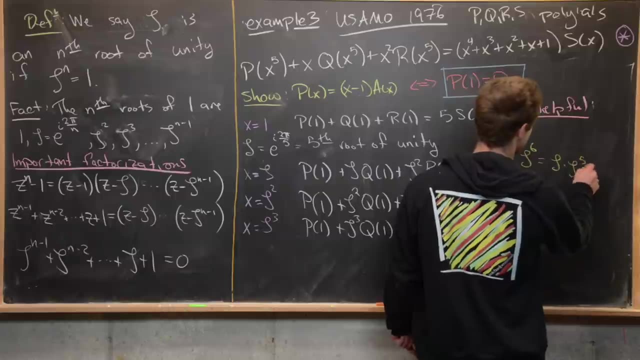 So that's equal to 1 plus zeta to the sixth. but what I want to notice over here is that zeta to the sixth is the same thing as zeta times zeta to the fifth, which is equal to zeta, because zeta to the fifth is equal to 1.. 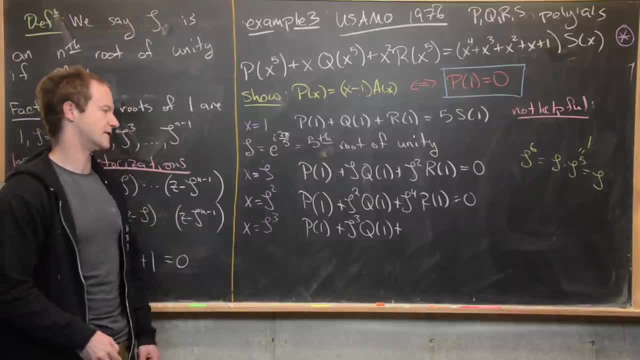 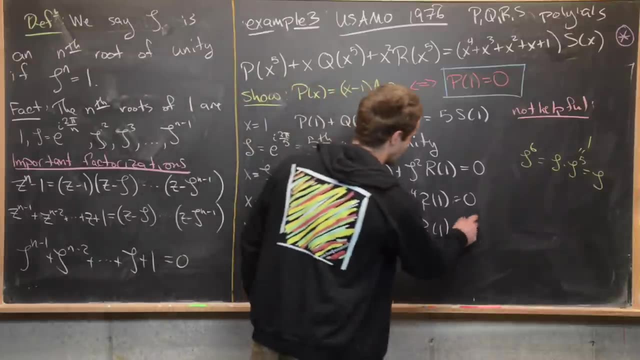 So in fact the exponents here are working modulo 5, if you want to think about it that way. So here we've got zeta times r to evaluate it at 1, and we have this is equal to 0. again, for the same reason. 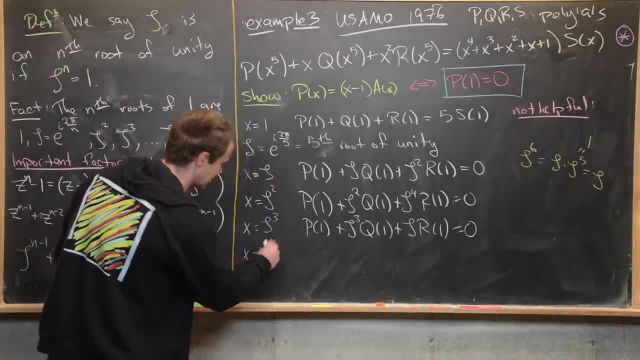 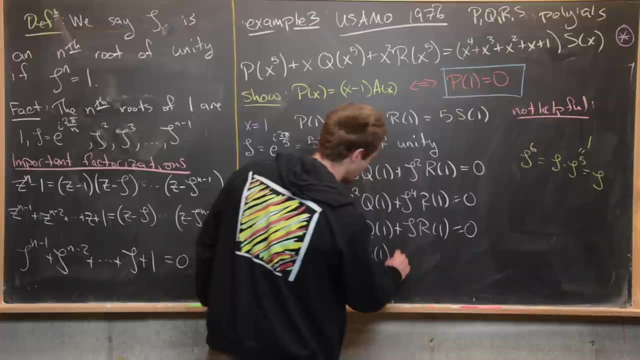 Now we've got 1.. We've got 1 more to check and that's x equals zeta to the fourth. So that's going to give us p of 1 plus zeta to the fourth, q of 1 plus zeta. 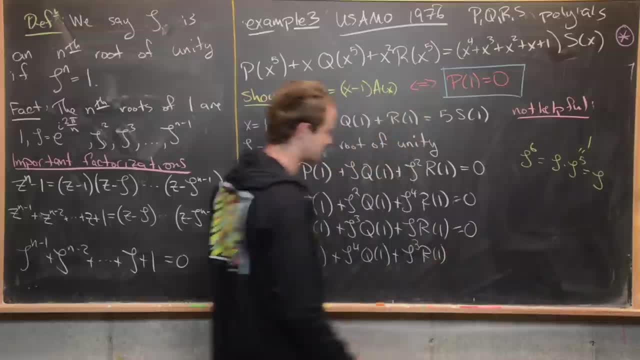 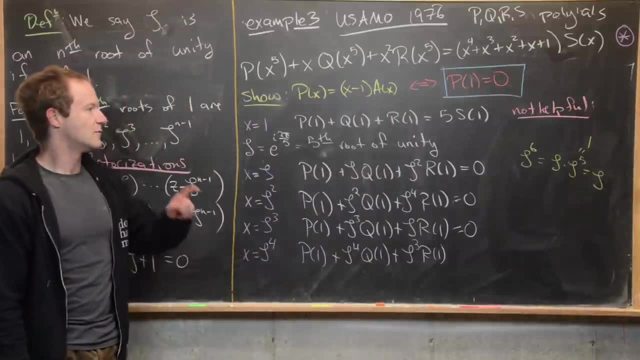 So this is going to be cubed r of 1. That's because we get zeta to the fourth squared, That's going to be zeta to the eighth. but we can reduce that using that trick over there to zeta cubed. 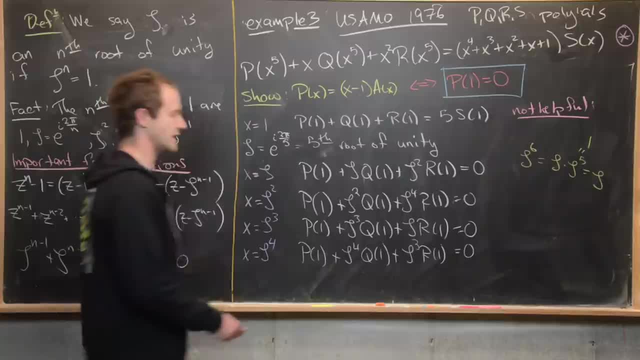 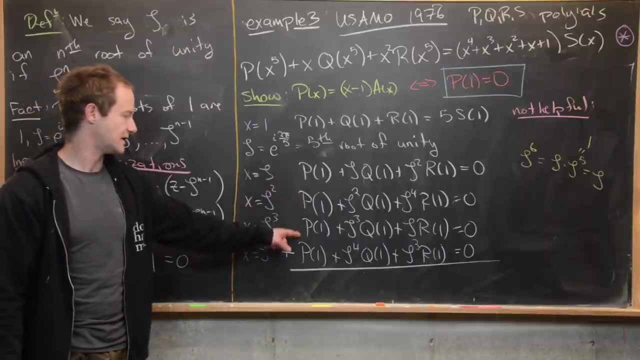 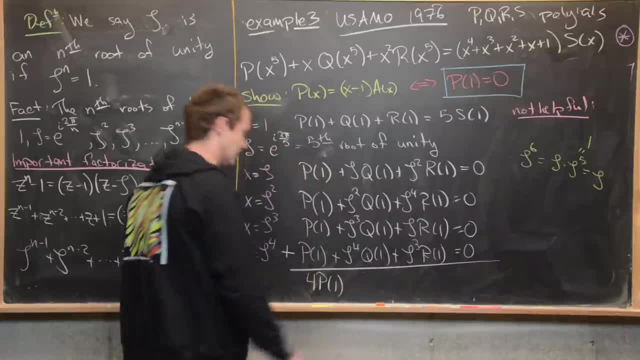 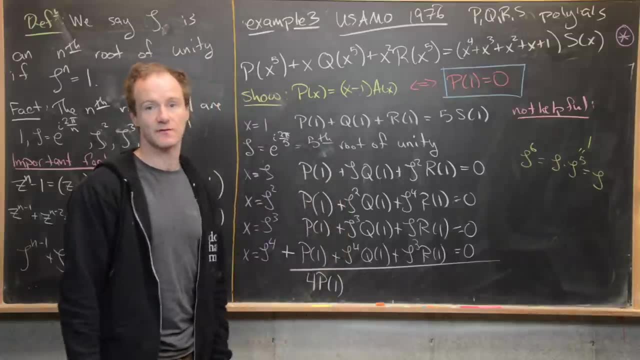 So notice that's going to be 4p evaluated at 1.. But now notice that adding up down here we have zeta plus zeta squared, plus zeta cubed, plus zeta to the fourth. But that's almost all of this. 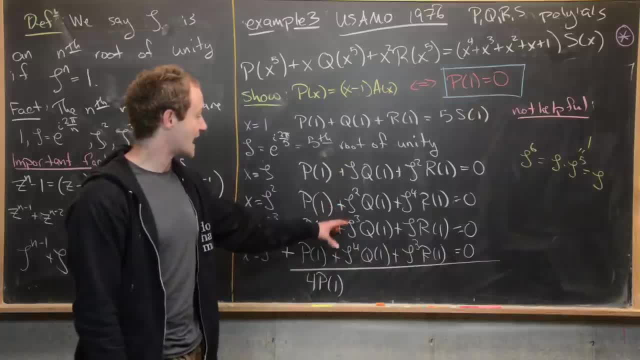 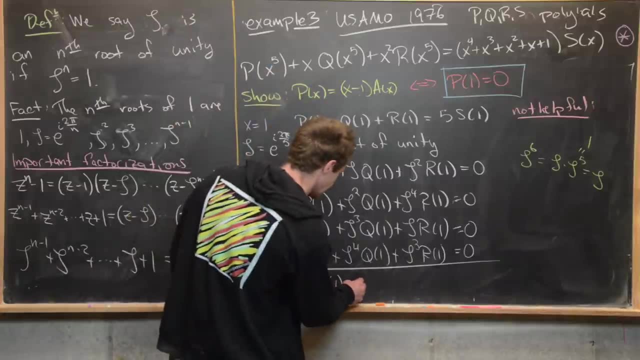 We're just missing a 1,, which means that if we add these up, we'll get a factor of minus 1.. Again, kind of by rule Rearranging this equation. So this is going to be minus q of 1.. 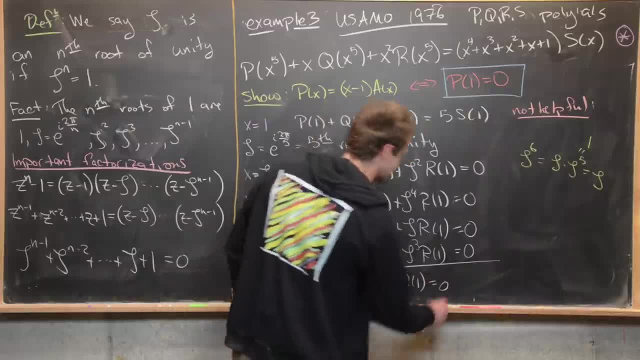 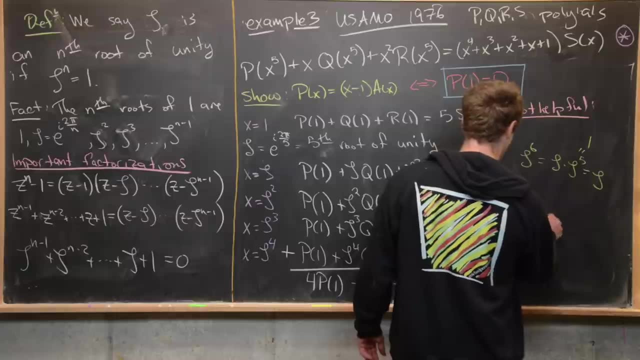 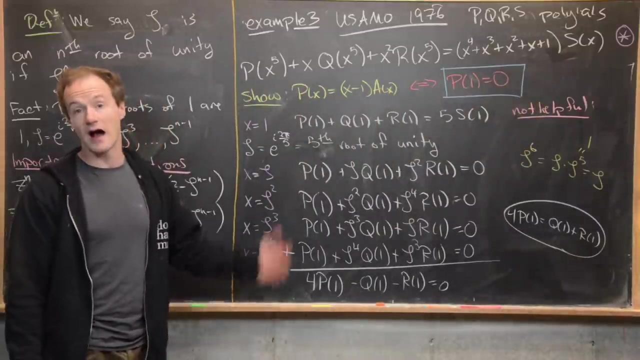 And then, similarly here we'll have: minus r of 1 equals 0.. Okay good, So that leaves us with this equation: 4 times p of 1 equals q of 1, plus r of 1.. And we're not quite done, but we've arrived at a useful equation. 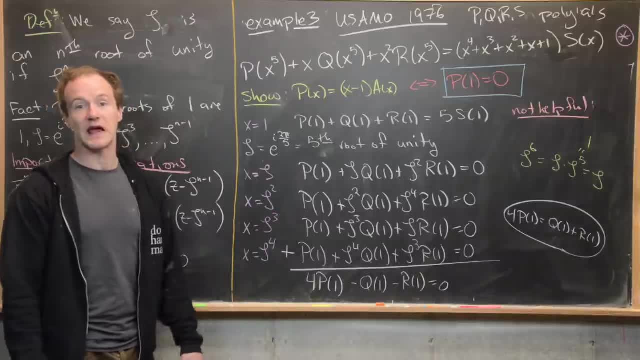 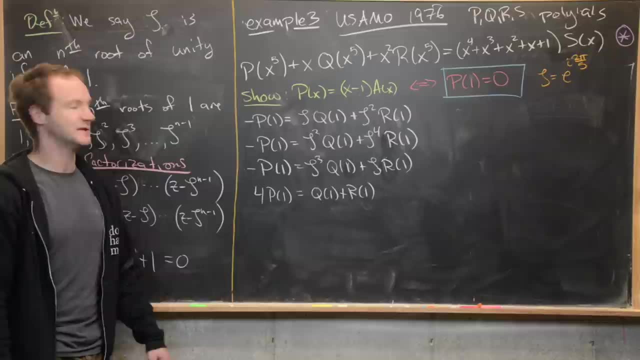 Okay, so I'm going to go ahead and clean up the board, keep what we need and then we'll finish it off. Okay, and the last board. We had this fifth root of unity, which we called zeta, And we arrived at some equations involving our polynomials evaluated at 1, along with these fifth roots of unity. 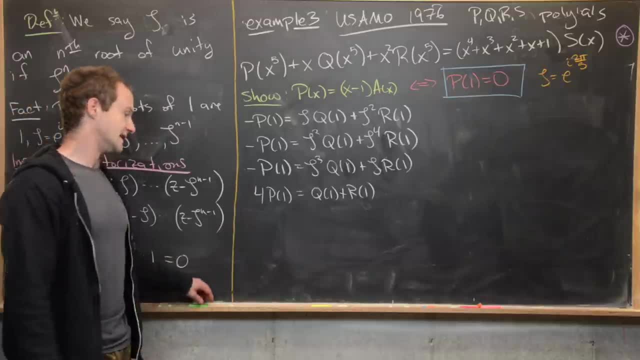 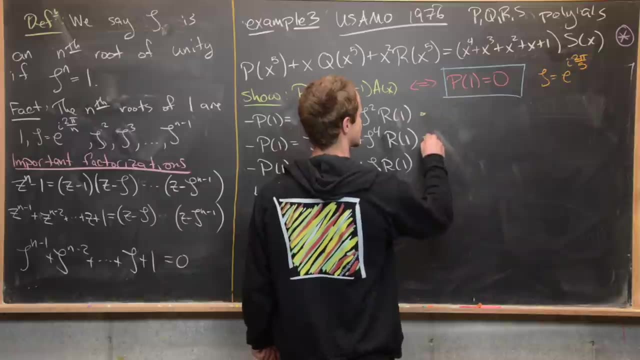 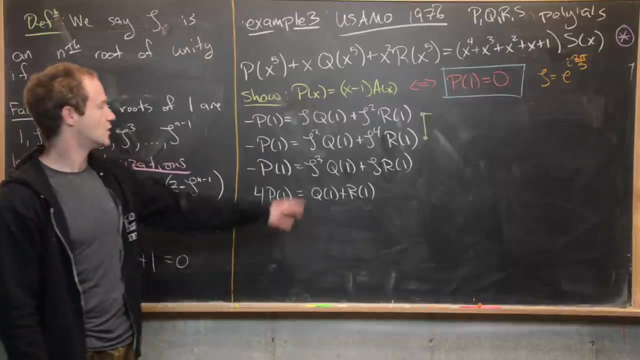 And so I've rewritten these a little bit, but it is equivalently what we had before. Okay, so first what I want to do is look at what these first two equations can give us. So let's take these first two equations And think about: minus p of 1 is equal to minus p of 1, which means this right-hand side equals this right-hand side. 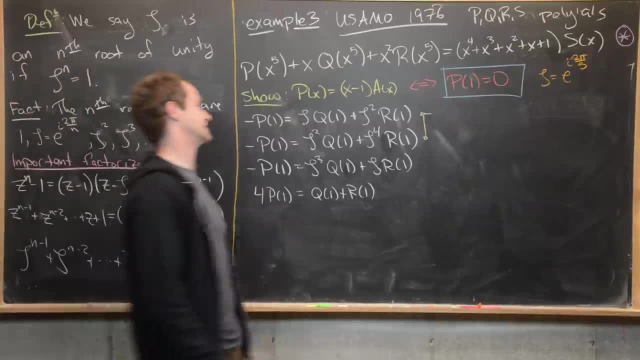 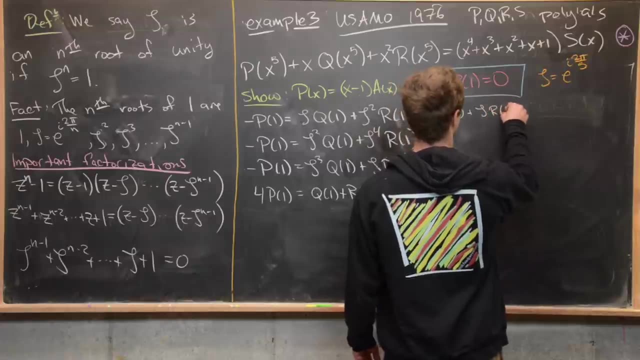 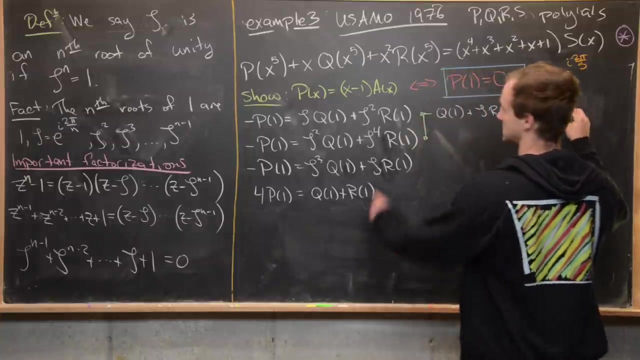 Both of these right-hand sides are multiples of zeta, so we can factor zeta out And that gives us this equation: q evaluated at 1 plus zeta times r evaluated at 1, equals zeta times q evaluated at 1 plus. 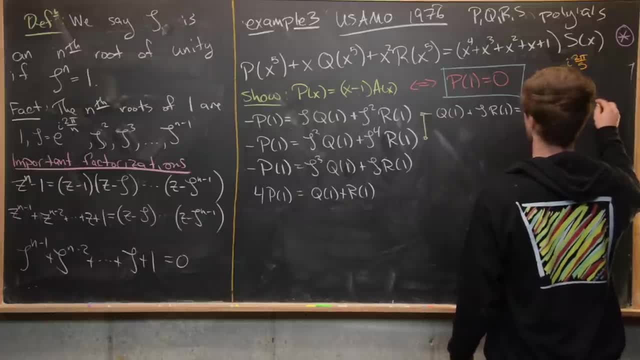 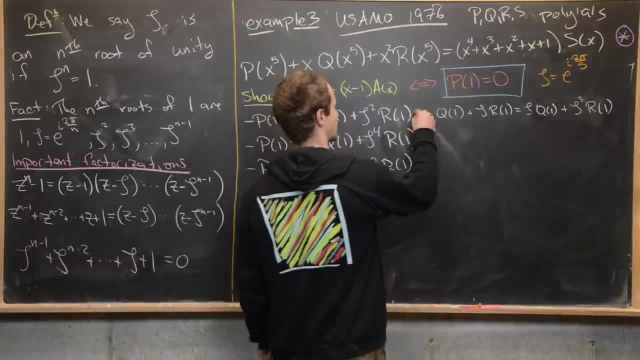 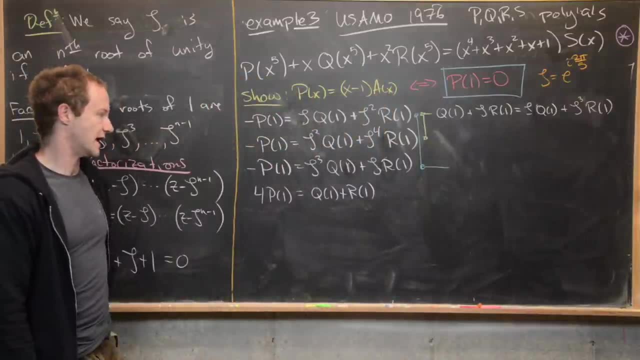 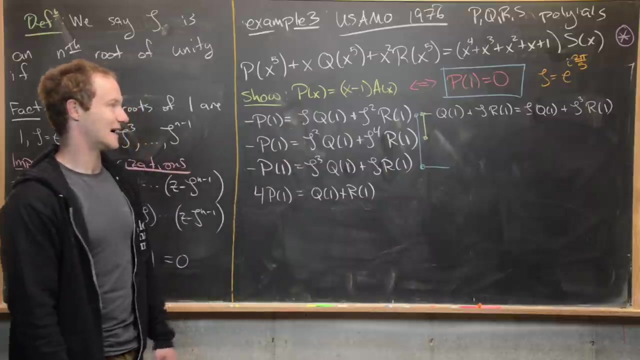 And then, likewise, we can do that with this first equation and this third equation, And that's going to give us another equation involving r1 and q1. Again, setting this minus p1 equal to this minus p1. And we can also factor zeta out, just like we did before. 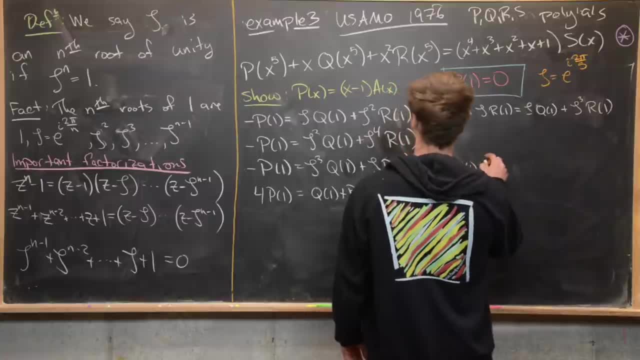 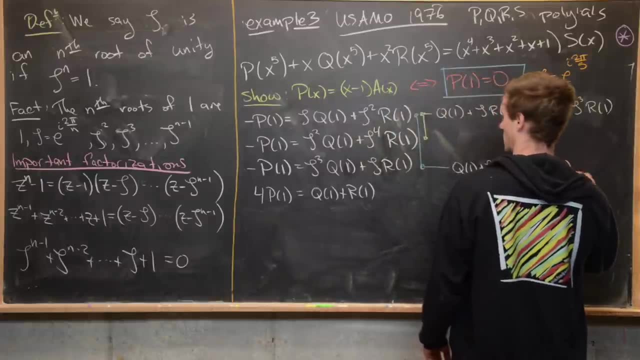 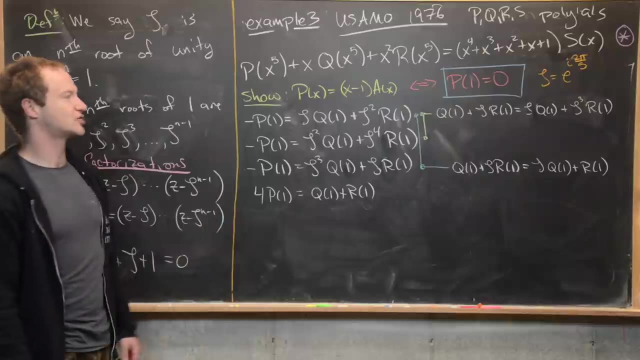 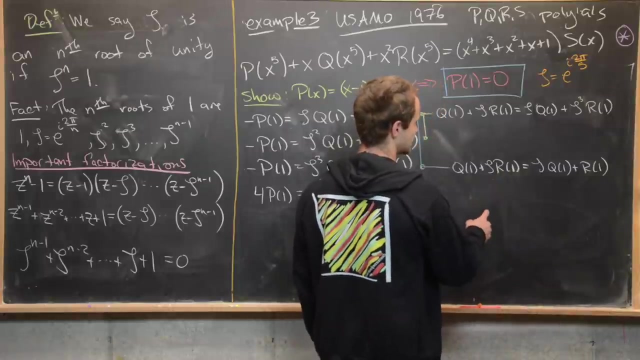 So notice, that's going to give us q1 plus zeta. zeta r1 equals zeta q1 plus r1, like that. Good. Now what I want to do is solve each of these for r. So let's see if we can do that. So notice, solving this one for r is not too bad. I can. 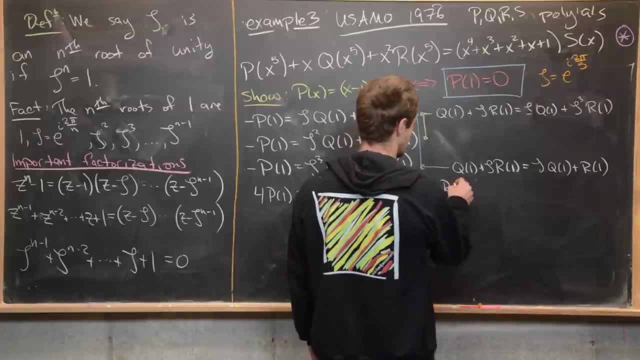 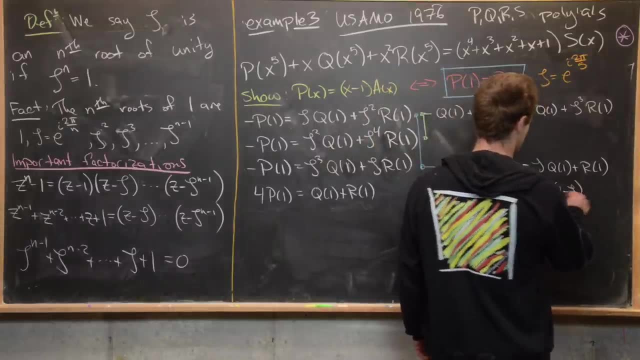 move this r over and this thing over. So that's going to give me r of 1 times 1 minus zeta, q of 1 times 1 minus zeta. Okay, well, that's pretty nice, because that tells us that r evaluated at. 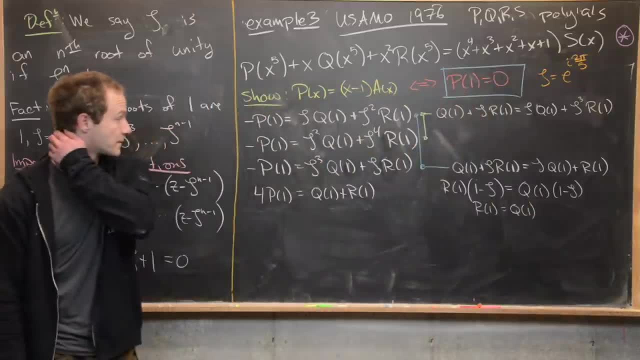 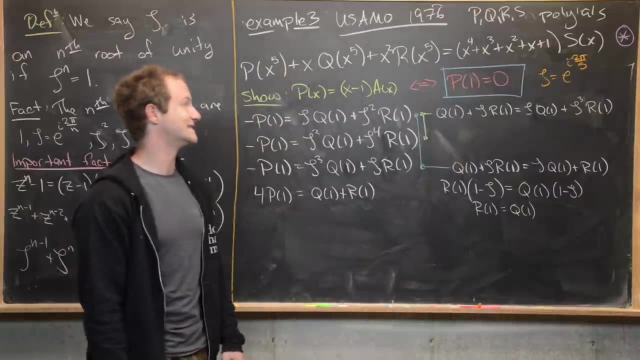 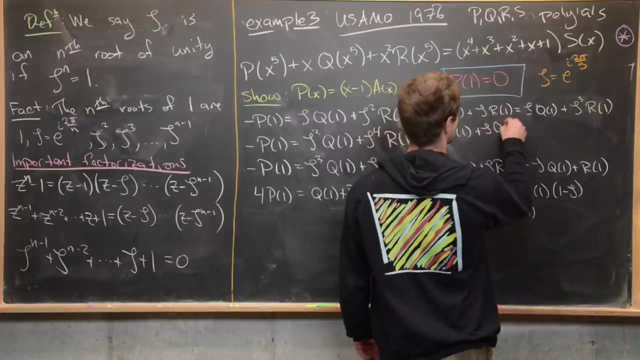 1 equals q, evaluated at 1.. Okay, so now we can plug r, evaluated at 1, equals q, evaluated at 1, into this equation And that's going to give us so q evaluated at 1 plus zeta times q evaluated at 1. 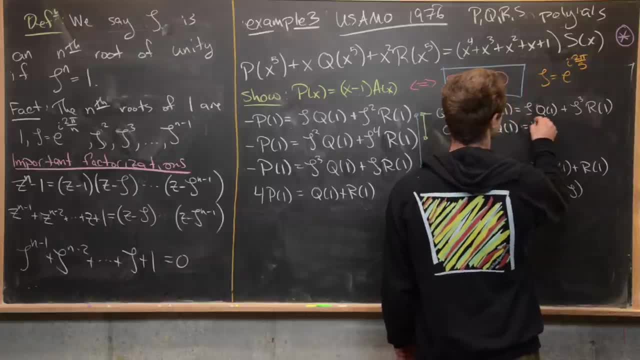 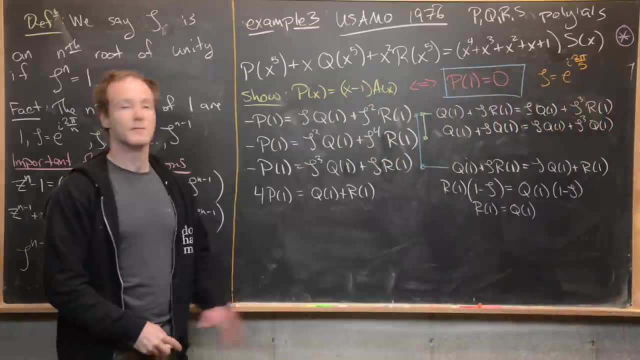 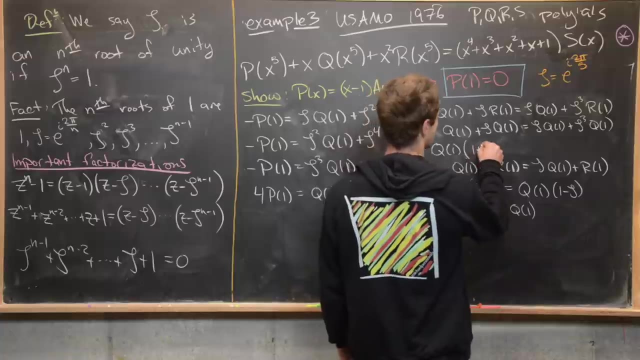 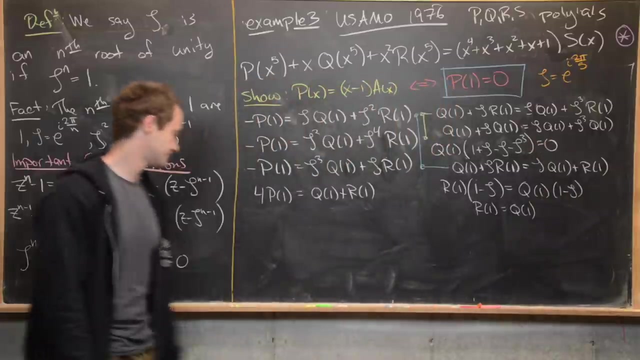 plus equals zeta times q, evaluated at 1, plus zeta cubed evaluated at q, evaluated at 1.. But now we can move everything over to one side of the equation And that'll give us something like q of 1 times the quantity 1 plus zeta minus zeta minus zeta cubed equals 0.. Good, But then we know as a fact this: 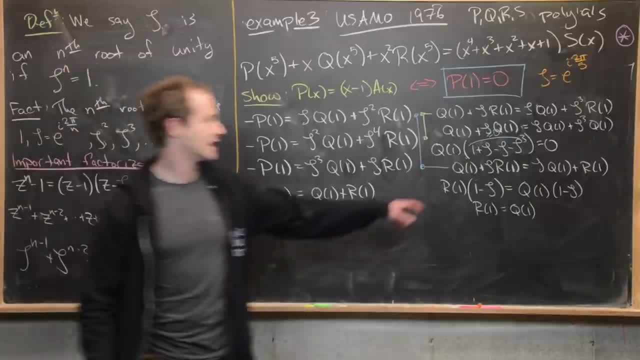 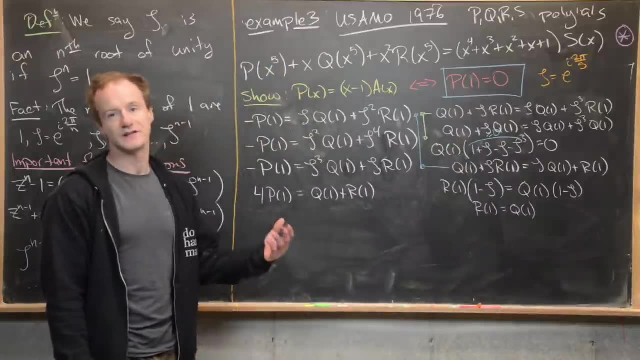 is not equal to 0. Again one. so we've got zeta minus zeta, So that is 0. But then we've got 1 minus zeta cubed. But we know zeta cubed is not equal to 1 because it's a fifth root of unity. So that means this thing: 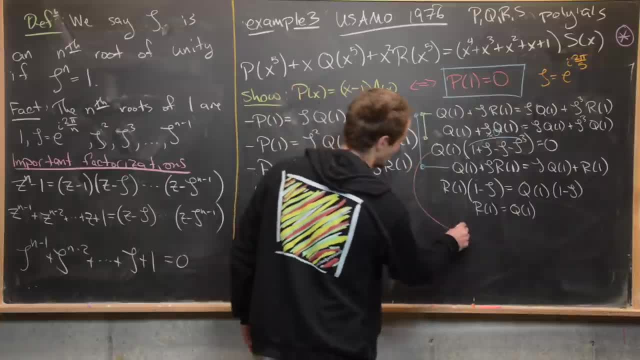 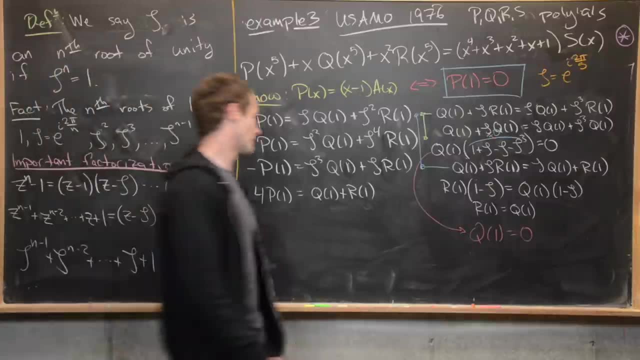 right here- is not equal to 0, which tells us that q must be equal to 0. So, sorry, q evaluated at 1 must be equal to 0. But then, likewise, r evaluated at 1 equals 0. But that means there's.